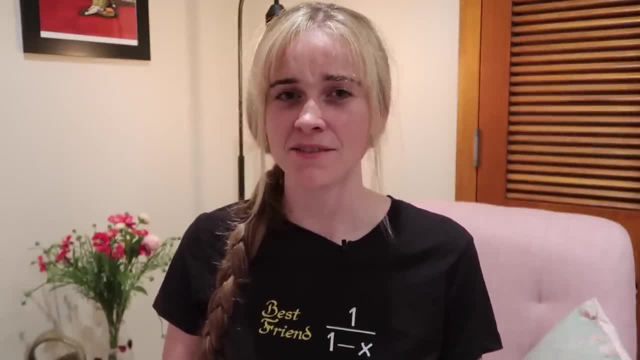 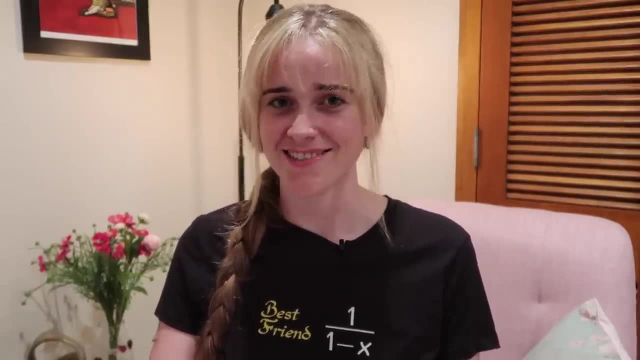 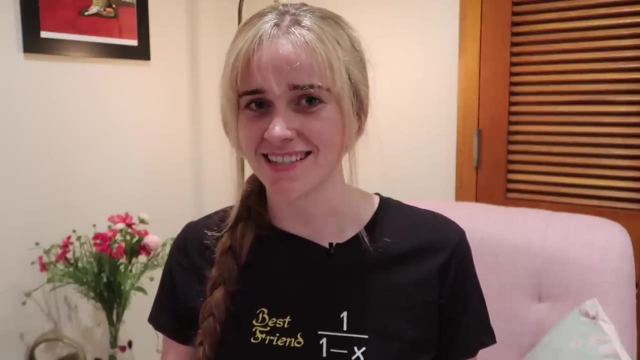 fare better on one of these tests just because the nature of them seems to involve a lot of like pattern recognition, with things like rotations, reflections, transformations- the same kind of things you might get really familiar with If you're doing a lot of geometry stuff in math. But regardless, through this video I'm going to 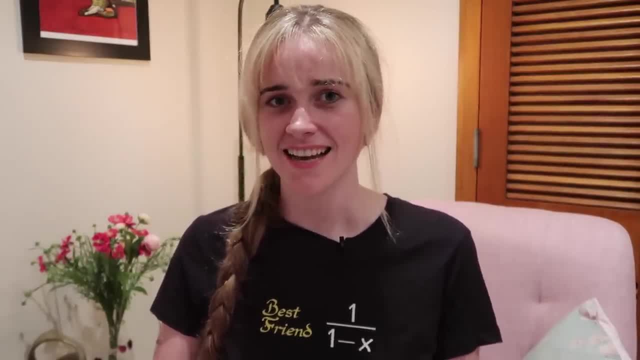 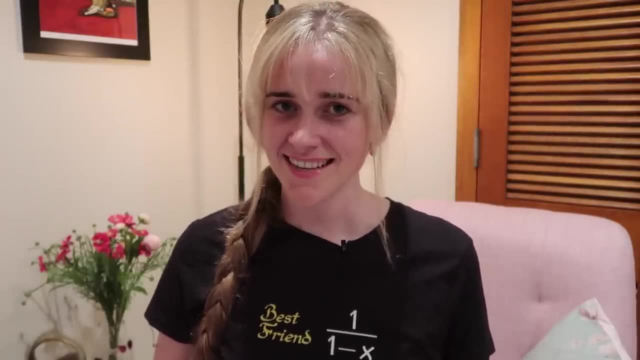 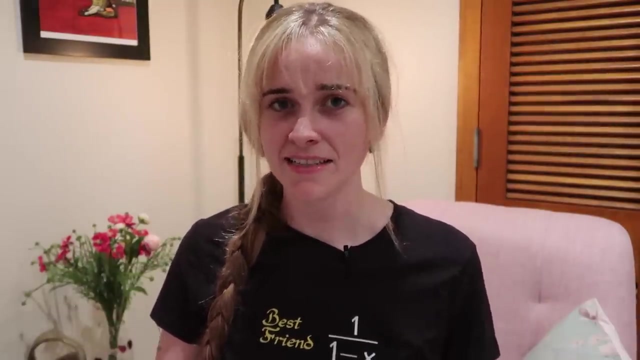 show you how a lot of these problems are supposed to be worked out, and maybe that will provide a few little hints or tricks on how to identify patterns. Now, Mensa is an organization that I guess is for people with really high IQ, So to get into Mensa you need to have scored in the top two percent. 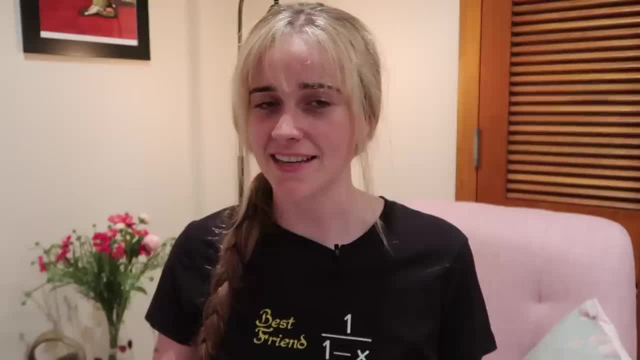 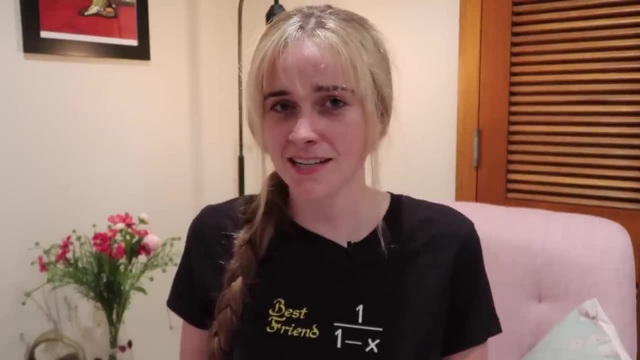 of the population on a score. So if you're doing a lot of geometry stuff in math, you're going to need a supervised IQ test, one that's officially recognized. I've heard that people in Mensa come from all walks of life. Some might be academics and some might have more ordinary jobs. The 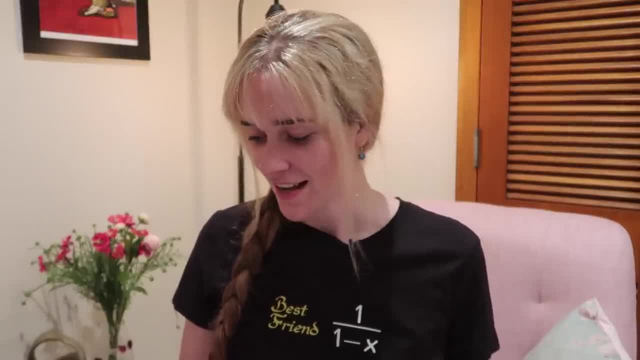 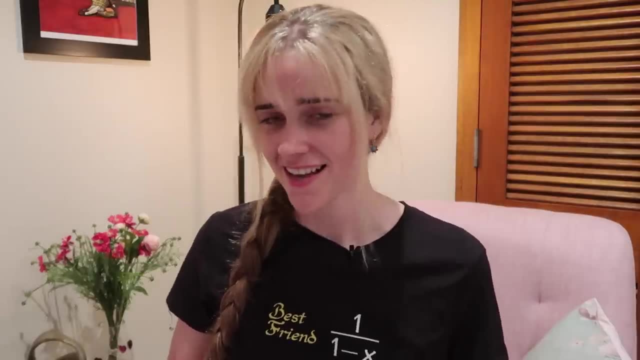 organization is not supposed to discriminate against anyone. They say on their website that they identify and foster human intelligence for the benefit of humanity. Maybe that sounds a little bit pretentious, I'm not sure, But today we're going to have a look at. 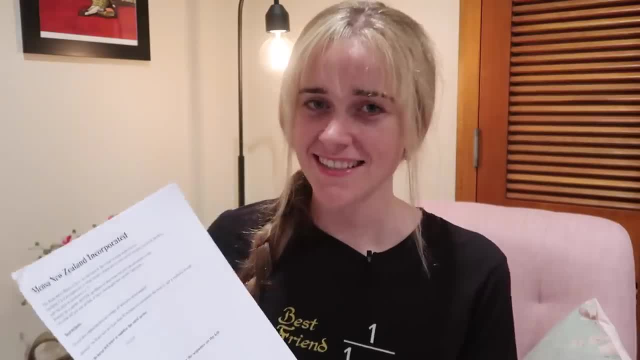 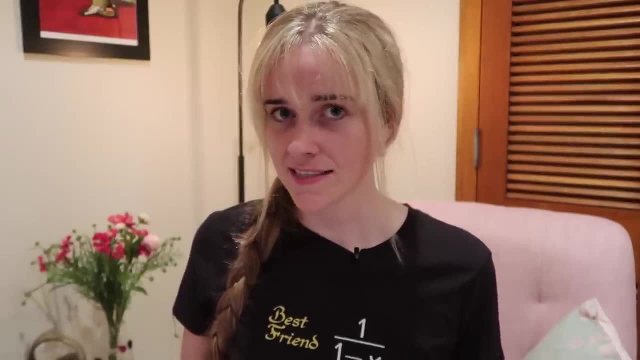 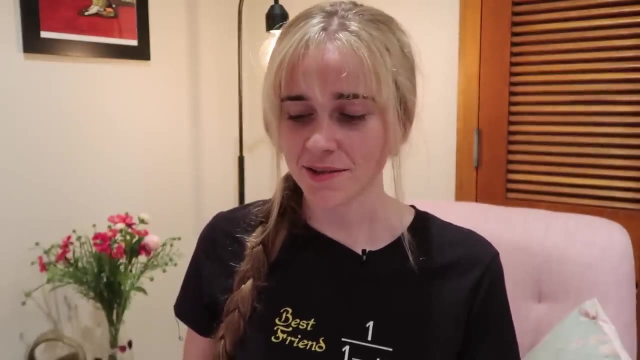 something that is a test from the New Zealand Mensa Society from their website, and the link will be in the description. This is an example of tests that people would need to take to get into Mensa and it's supposed to give an idea of you know what kind of questions you could expect. 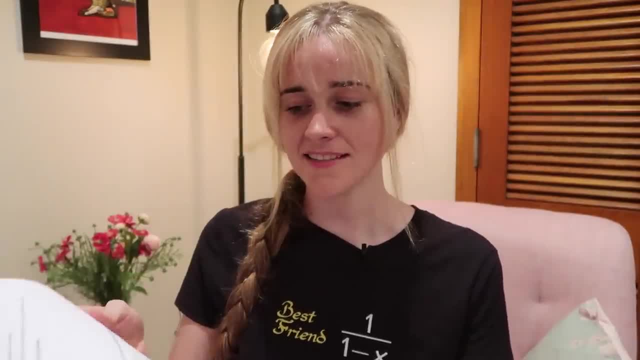 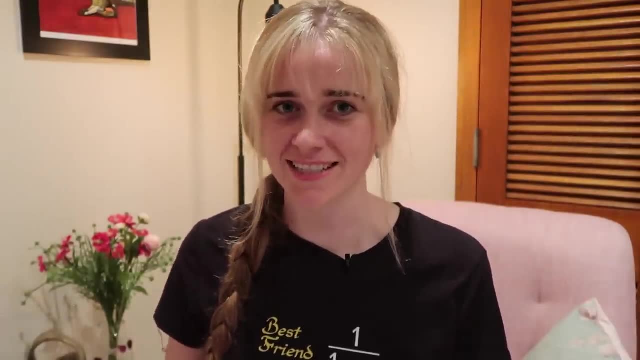 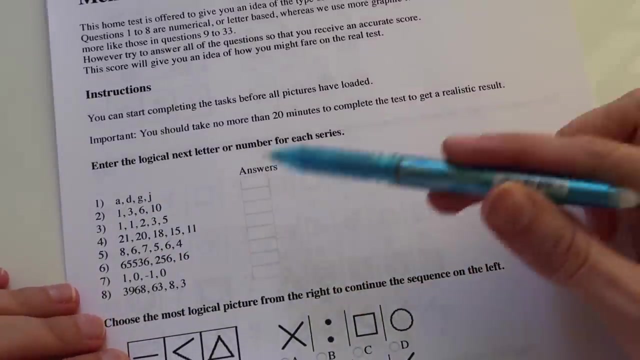 This test is supposed to take no more than 20 minutes and I'd advise- maybe you want to have a little try of it yourself- by following the link before I start explaining some of the answers. This test starts off with some letter and number based questions, but it says that these type of 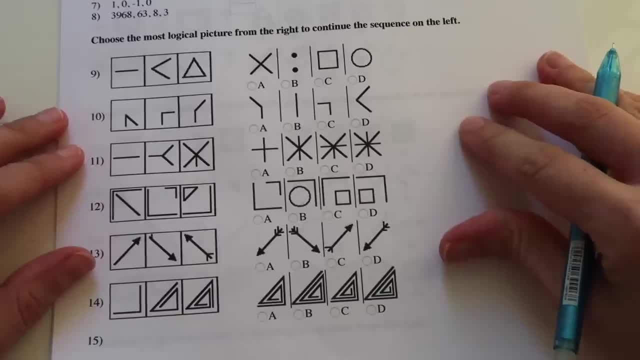 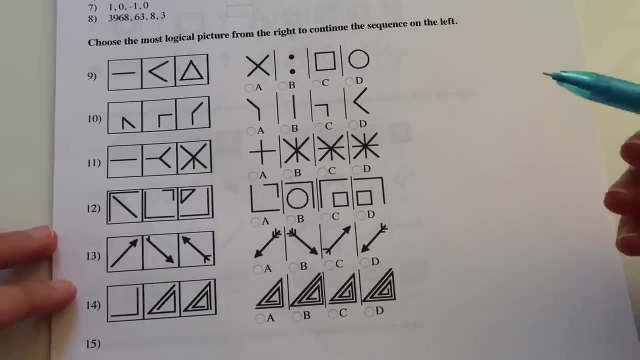 questions are being phased out, so we're just going to look at the more visual questions, And I have already tried the test for myself and had a look at the answers they provide, so I'm giving you insight into how you're supposed to solve these. I'll have time to go through a few in every section. 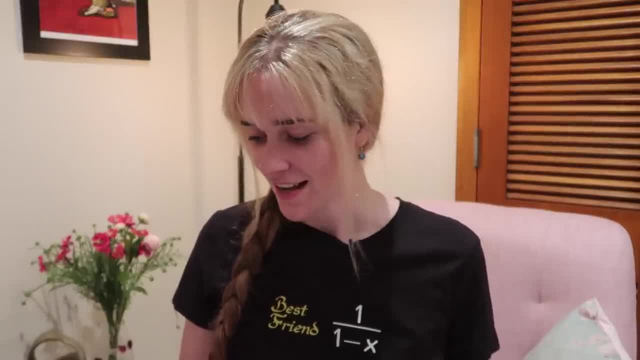 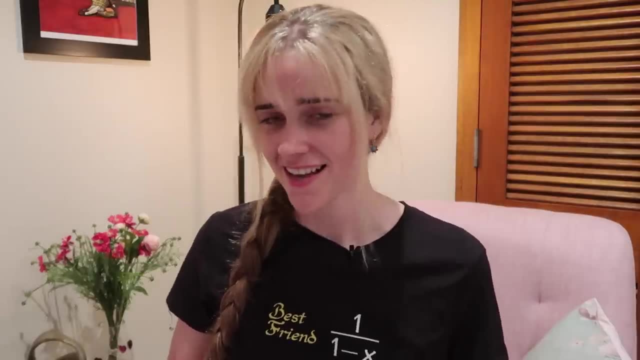 organization is not supposed to discriminate against anyone. They say on their website that they identify and foster human intelligence for the benefit of humanity. Maybe that sounds a little bit pretentious, I'm not sure, But today we're going to have a look at. 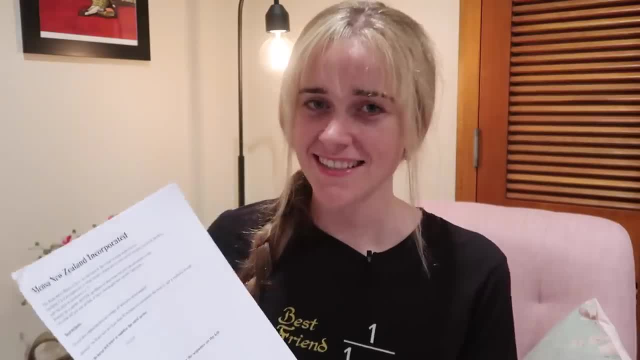 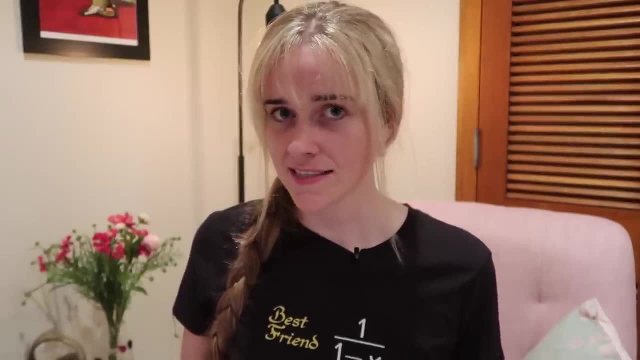 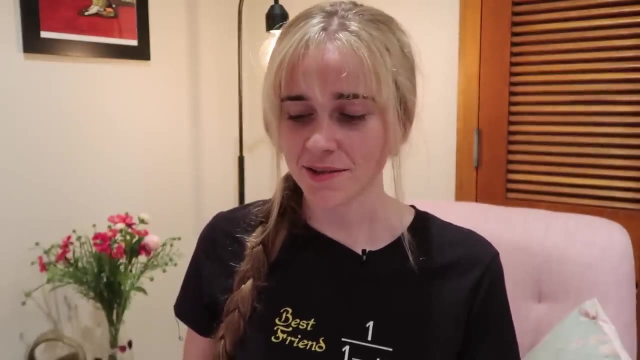 something that is a test from the New Zealand Mensa Society from their website, and the link will be in the description. This is an example of tests that people would need to take to get into Mensa and it's supposed to give an idea of you know what kind of questions you could expect. 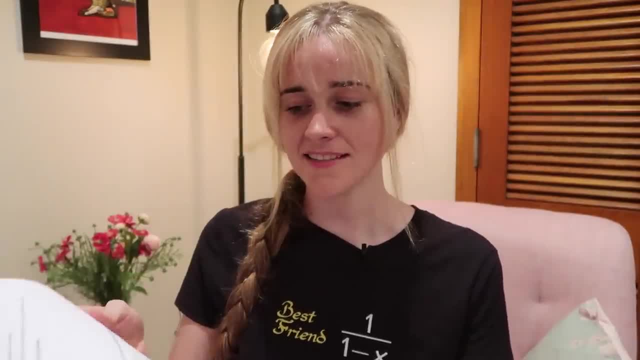 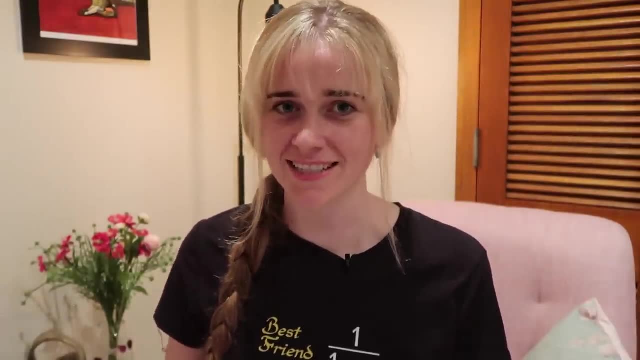 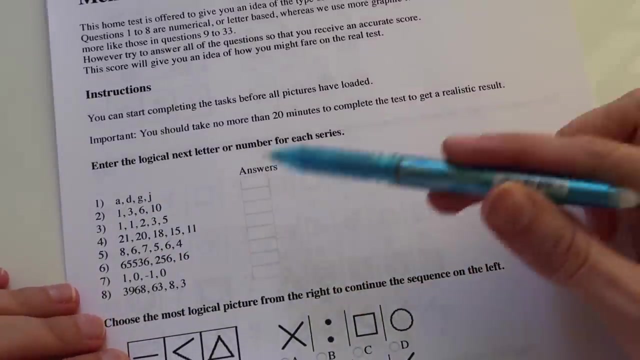 This test is supposed to take no more than 20 minutes and I'd advise- maybe you want to have a little try of it yourself- by following the link before I start explaining some of the answers. This test starts off with some letter and number based questions, but it says that these type of 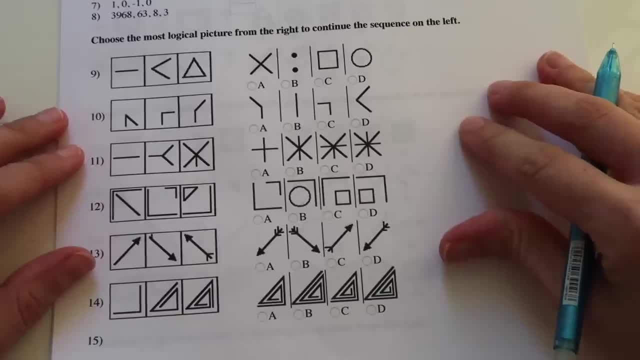 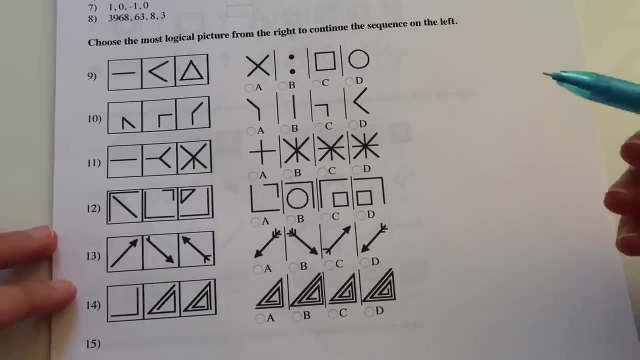 questions are being phased out, so we're just going to look at the more visual questions, And I have already tried the test for myself and had a look at the answers they provide, so I'm giving you insight into how you're supposed to solve these. I'll have time to go through a few in every section. 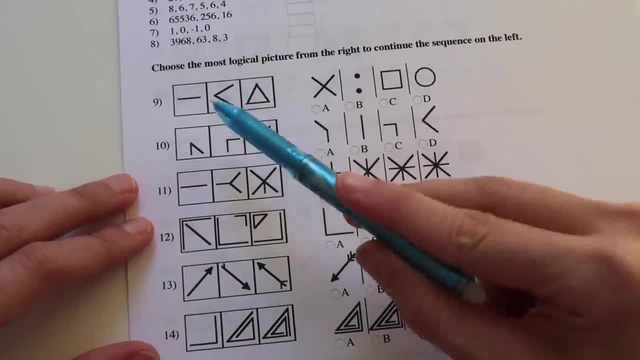 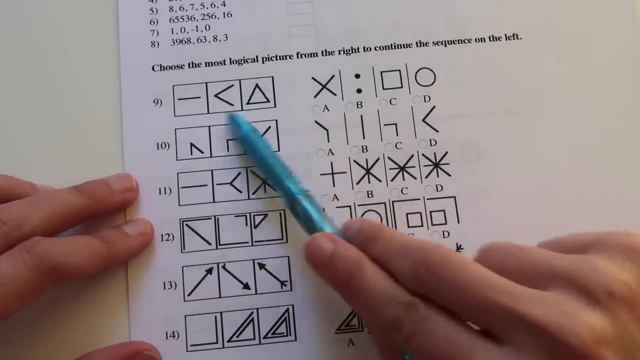 but I won't be solving every problem here. If we look at the first one, we're being asked to choose the most logical picture from the right to continue the sequence on the left. So we need to look at this and set up some pattern that's happening. At first glance, they just look like three random different shapes and 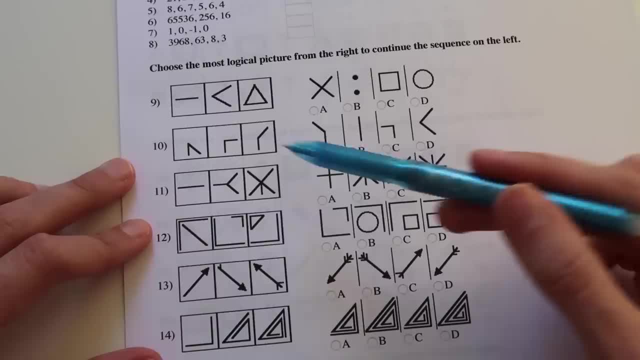 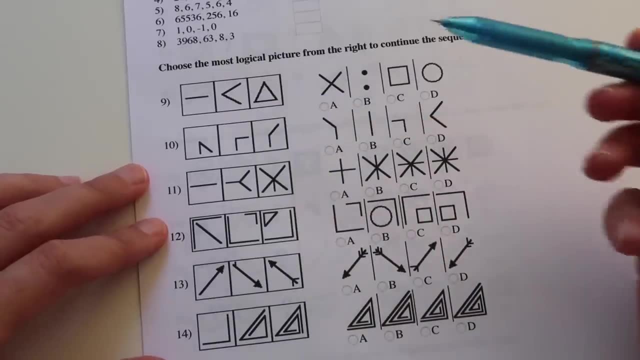 you might be tempted to just randomly pick an answer that you feel looks good sitting next to those, But try and think about the properties of these shapes. What's actually going on? Well, one property of shapes is the number of sides that it has. So here we have just one side or one line. 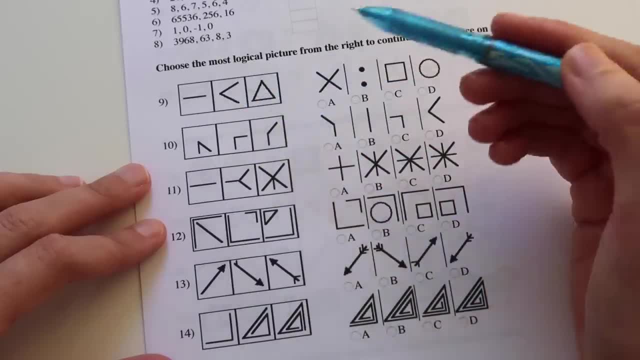 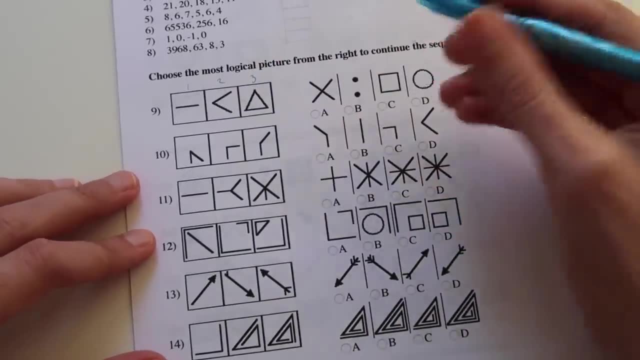 This shape would have two sides and three, So that gives us a pattern of one, two, three, meaning we should look for a shape with four sides and there's just one of those C A kind of has four lines coming out of the center, but it's actually. 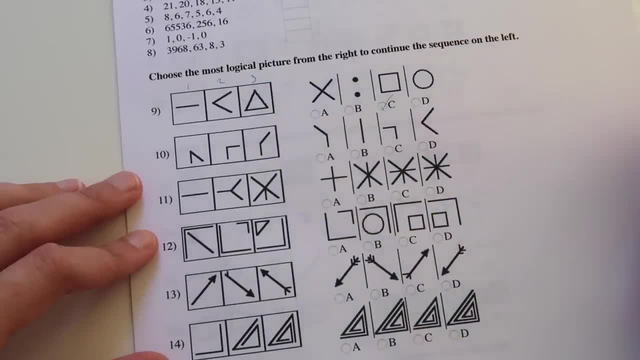 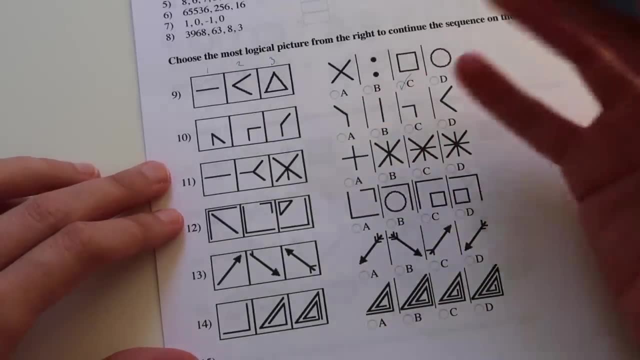 the number of sides, not lines coming out of the center, otherwise three wouldn't fit. So that gives us C. Looking at number 10, try to figure out. you know what's staying the same and what's changing throughout. If we look at this, we see this line on the bottom. looks like a bit of a clock, The little. 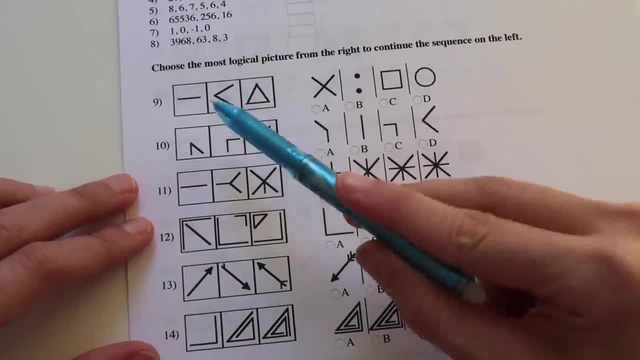 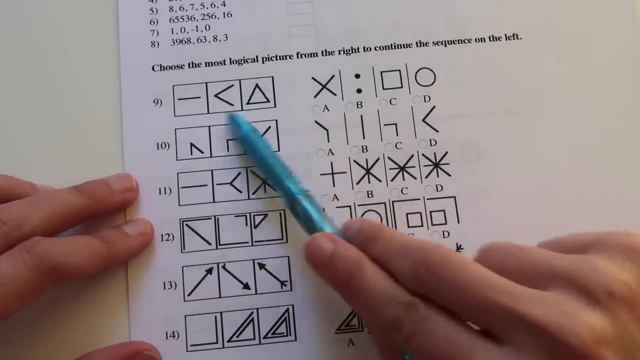 but I won't be solving every problem here. If we look at the first one, we're being asked to choose the most logical picture from the right to continue the sequence on the left. So we need to look at this and set up some pattern that's happening. At first glance, they just look like three random different shapes and 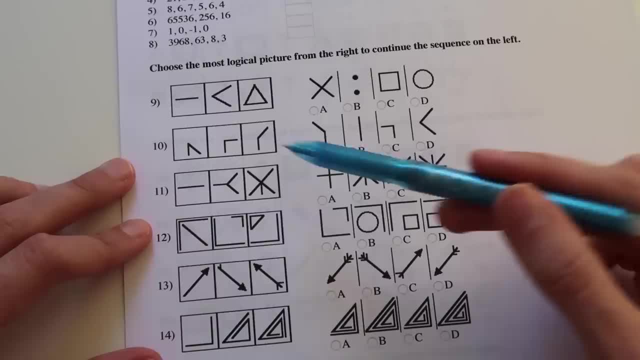 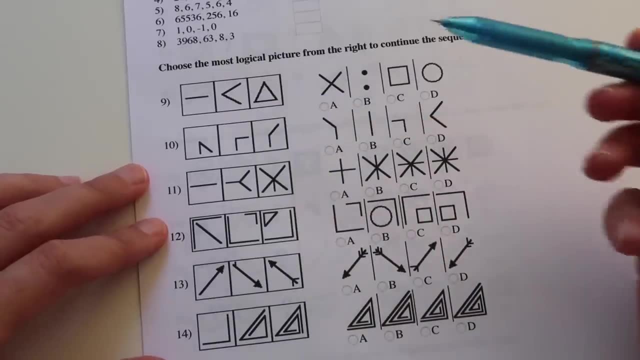 you might be tempted to just randomly pick an answer that you feel looks good sitting next to those, But try and think about the properties of these shapes. What's actually going on? Well, one property of shapes is the number of sides that it has. So here we have just one side or one line. 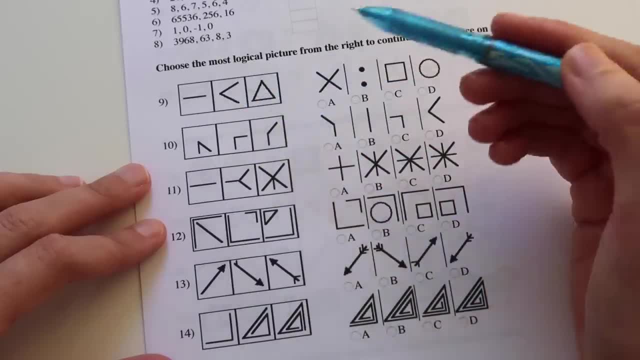 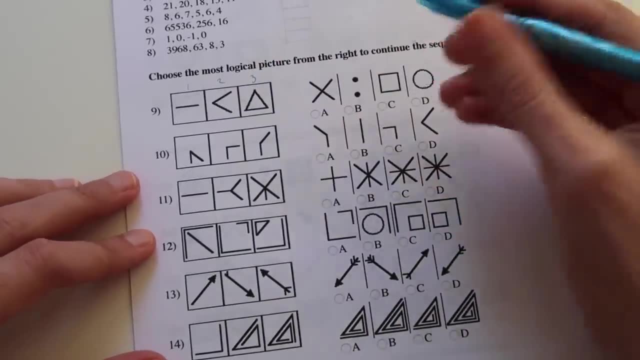 This shape would have two sides and three, So that gives us a pattern of one, two, three, meaning we should look for a shape with four sides and there's just one of those C A kind of has four lines coming out of the center, but it's actually. 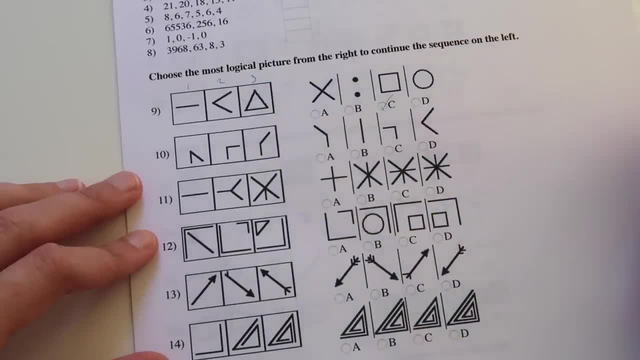 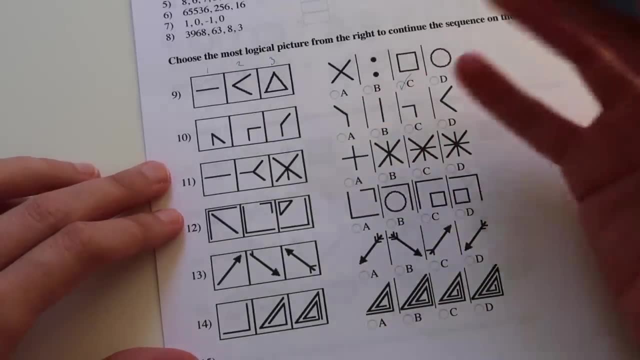 the number of sides, not lines coming out of the center, otherwise three wouldn't fit. So that gives us C. Looking at number 10, try to figure out. you know what's staying the same and what's changing throughout. If we look at this, we see this line on the bottom. looks like a bit of a clock, The little. 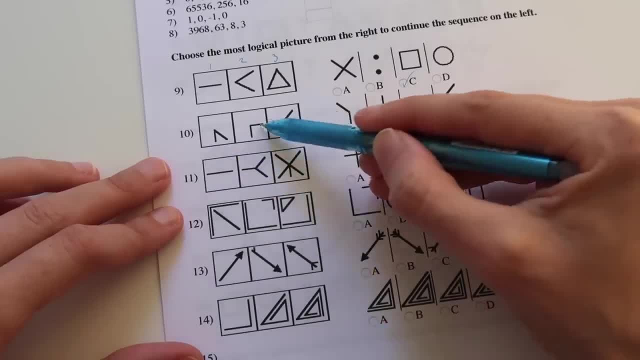 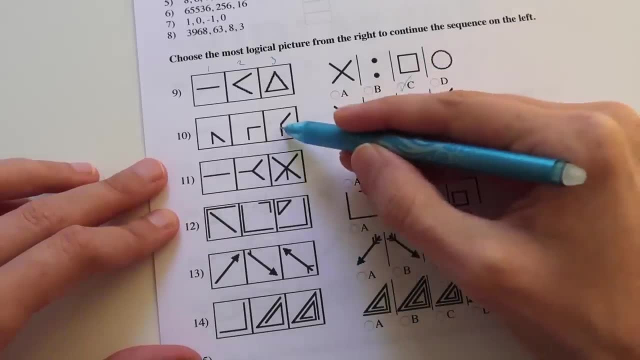 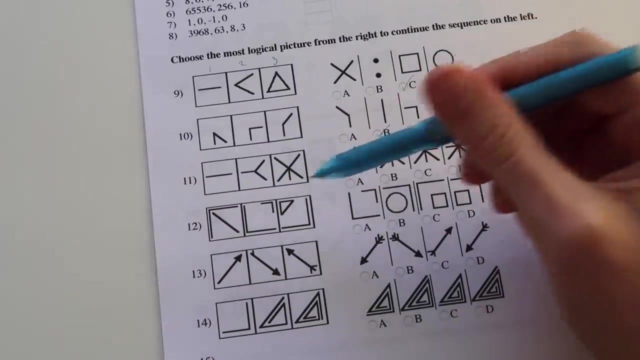 line down here is staying on six and this hand is moving around counterclockwise around the clock, meaning that by the time we get to the next in the sequence, we'd expect this hand to still be on the bottom and this one will have moved to be straight. So that would give us B. Number 11 shows: 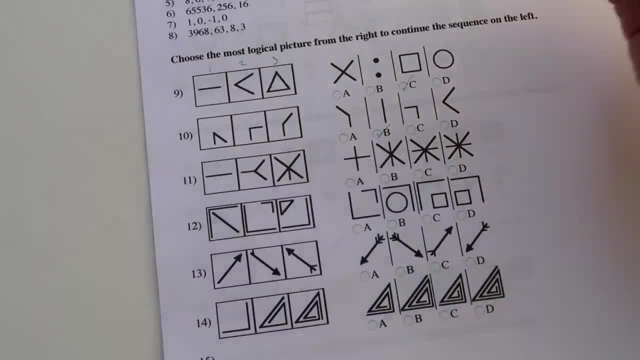 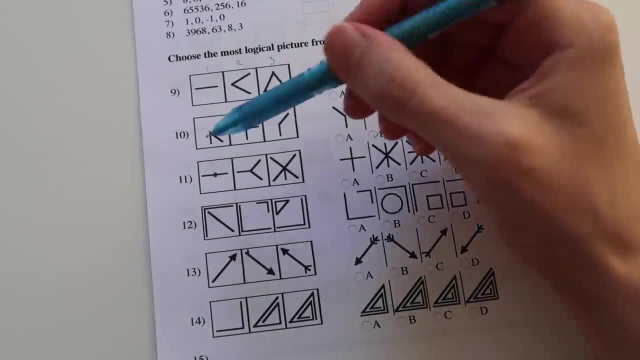 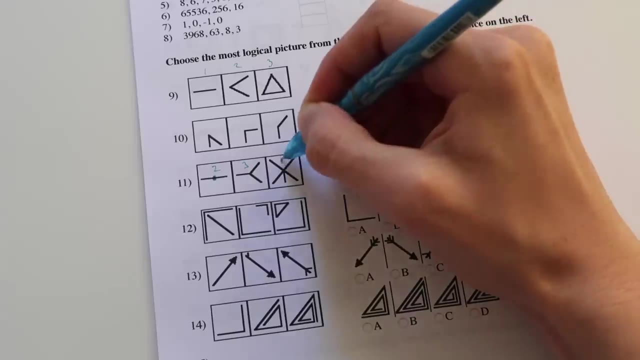 that sometimes you need to sort of pick a reference point. In this case it is establishing that the center of the image and lines coming out of the center are what we're going to care about. So in number 11 we have two lines coming out of the center and the next one three, five. What's the? 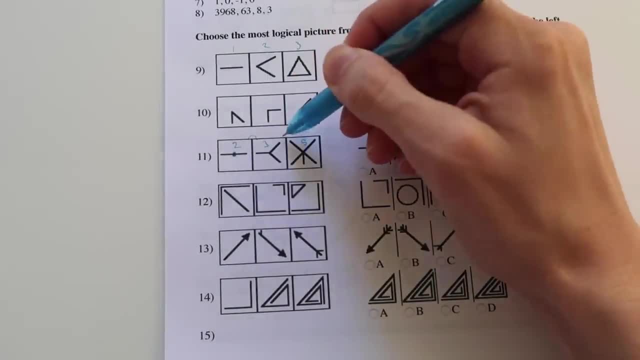 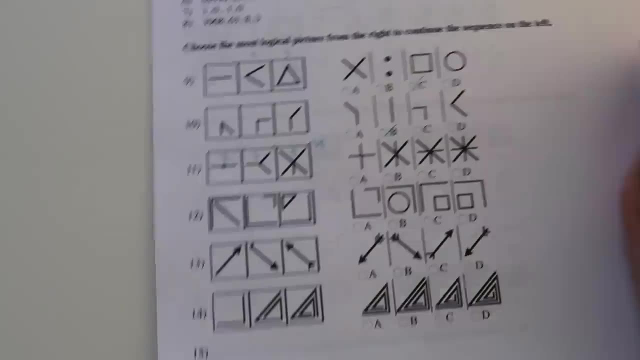 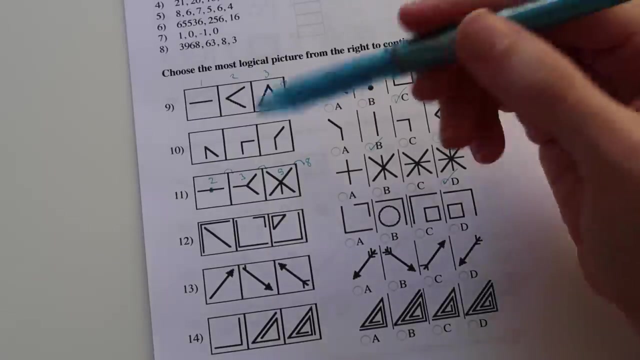 pattern between two, three and five. Well, this increases by one, this increases by two. We would expect an increase of three. So we'd expect something with eight lines coming out of the center, and D gives us that answer. Number 11. when I did on my own, I got a different answer. I was: 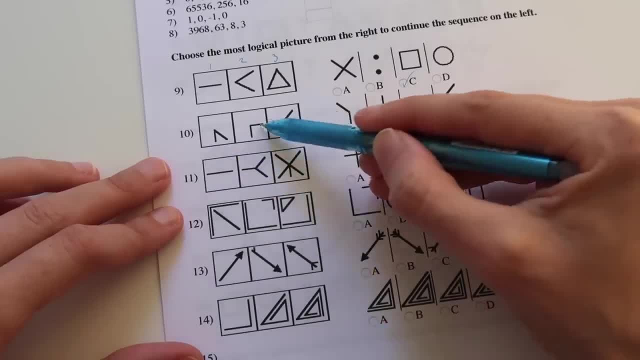 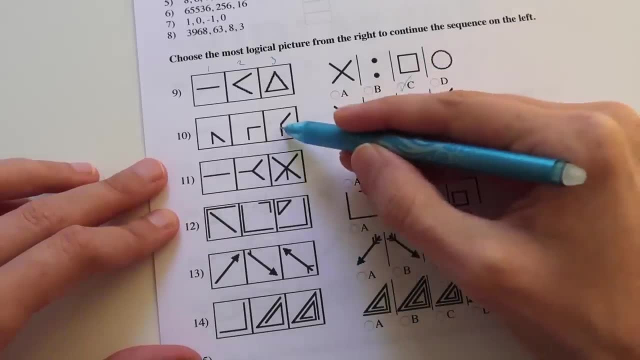 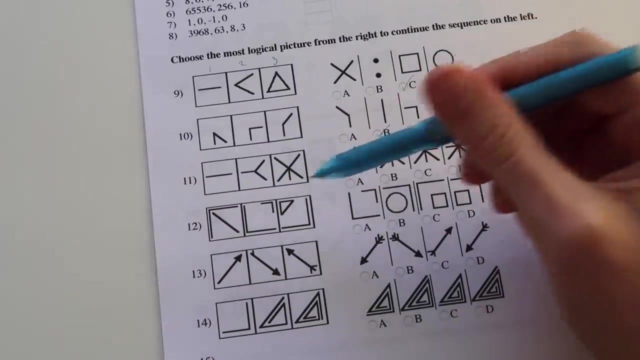 one down here is staying on six and this hand is moving around counterclockwise around the clock, meaning that by the time we get to the next in the sequence, we'd expect this hand to still be on the bottom and this one will have moved to be straight. So that would give us B. Number 11 shows: 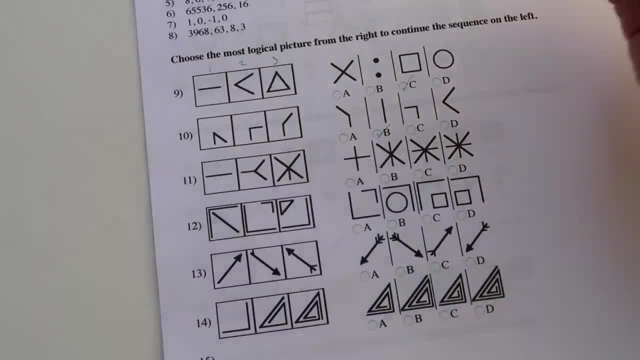 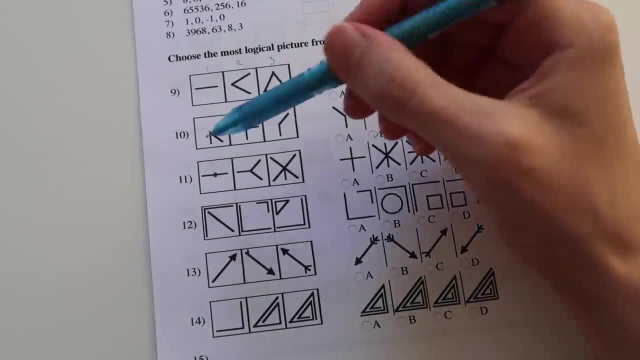 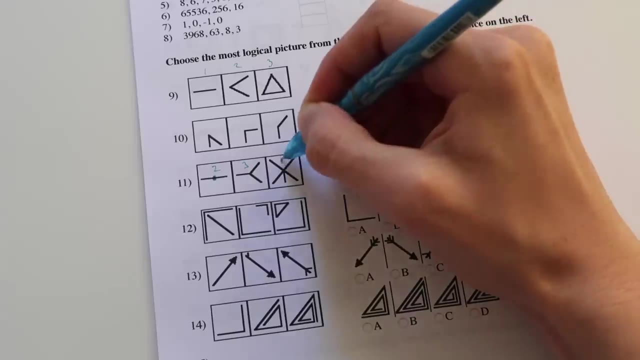 that sometimes you need to sort of pick a reference point. In this case it is establishing that the center of the image and lines coming out of the center are what we're going to care about. So in number 11 we have two lines coming out of the center and the next one three, five. What's the? 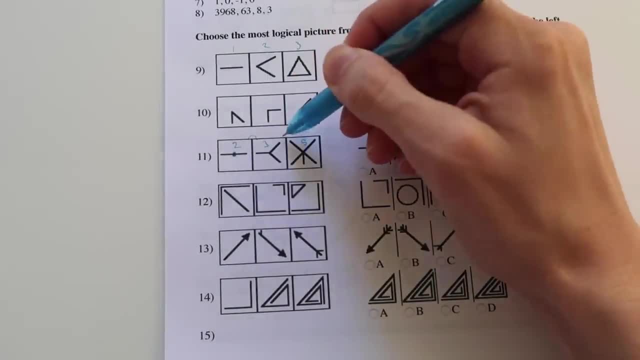 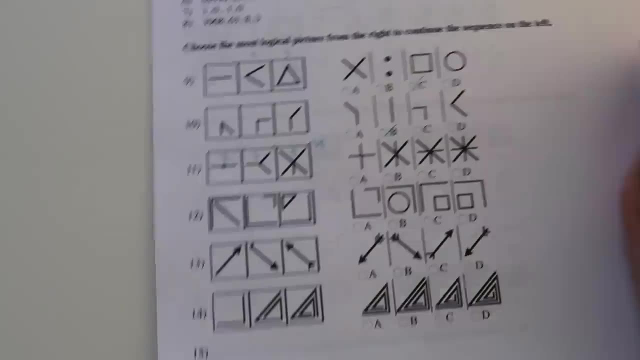 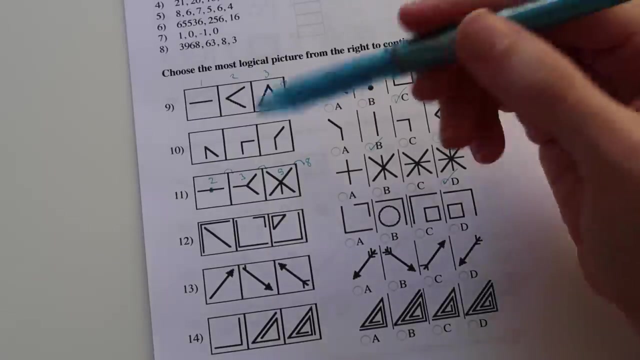 pattern between two, three and five. Well, this increases by one, this increases by two. We would expect an increase of three. So we'd expect something with eight lines coming out of the center, and D gives us that answer. Number 11. when I did on my own, I got a different answer. I was: 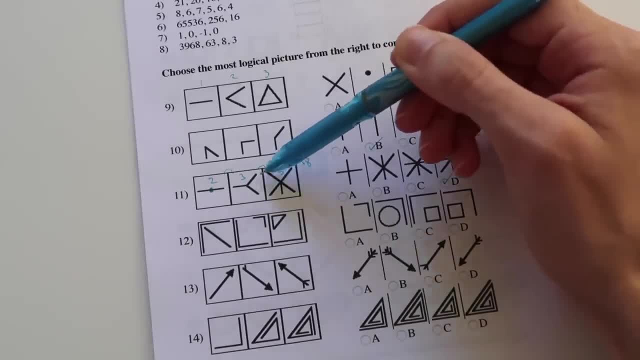 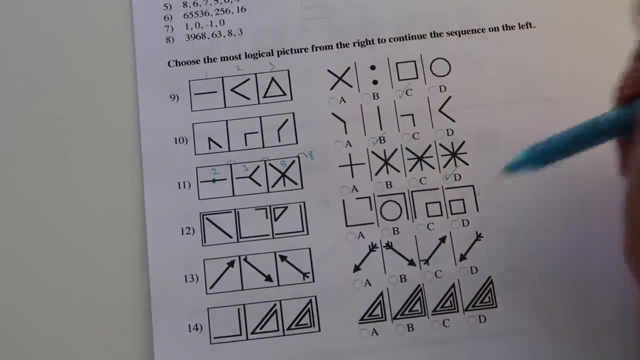 thinking that, oh, we're adding this V shape on every time, So you've added it here and then we've added it in here. If you added a V shape onto this one, you'd get C, but the answer that they give is D, and I agree that's a better way to do it. The rest of these problems are very similar. You're just 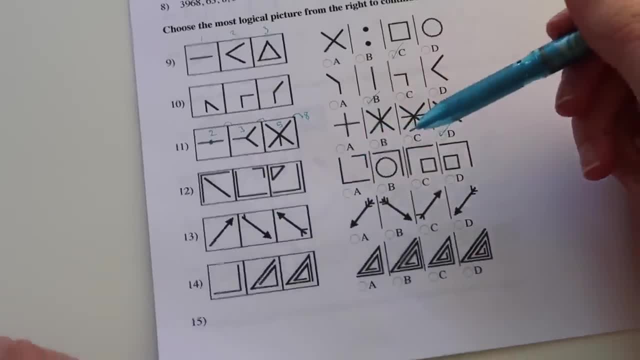 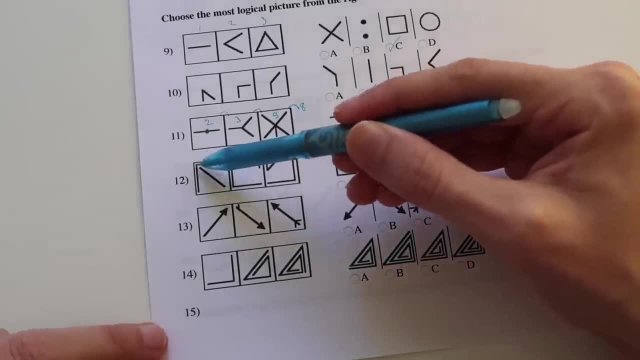 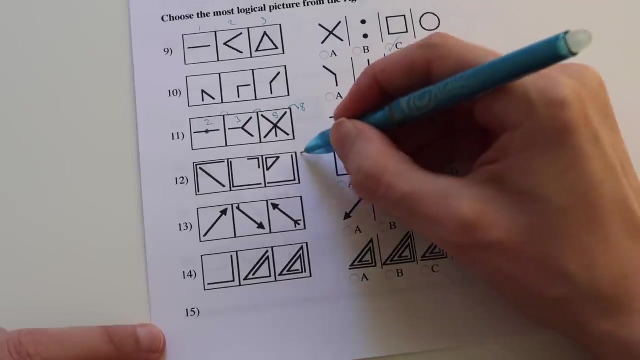 looking for, like slight changes or ways that these pictures evolve that are consistent. Sometimes different elements in the pictures evolve differently to other elements. like for number 12, we have this L which is going around the outside of the square counterclockwise, so we'd expect to. 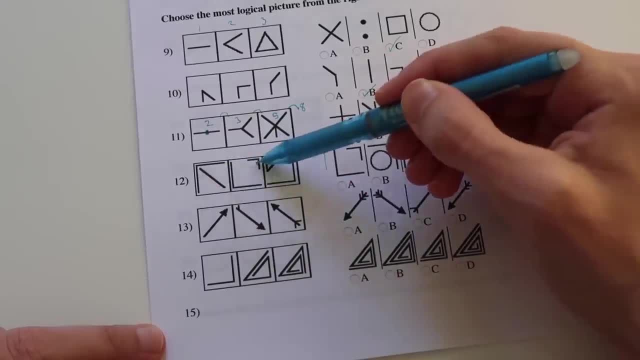 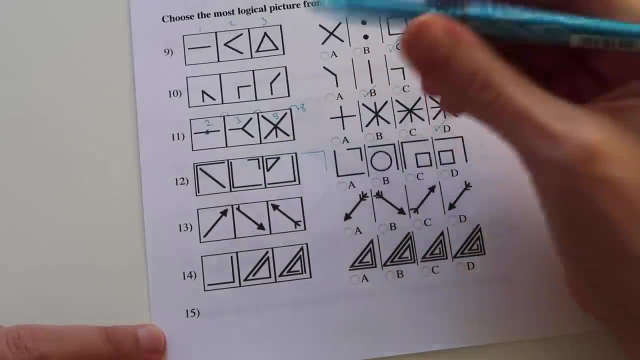 have a line like that in the next one and that's sort of independent from what's happening to the shape in here, which is that in like number nine the shape is increasing inside one every time. So we'd expect a square in the next one and a square and a line like that. that would give us D. 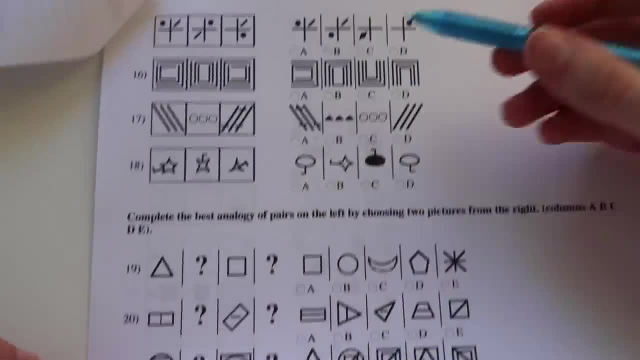 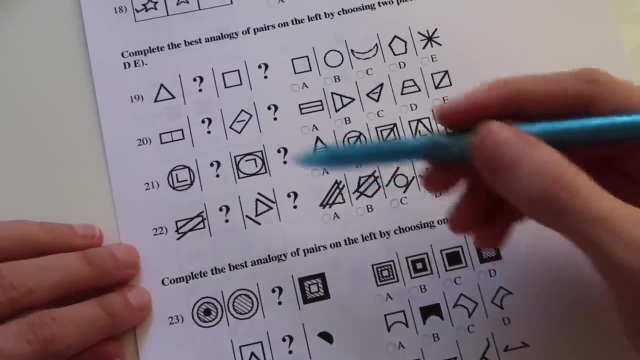 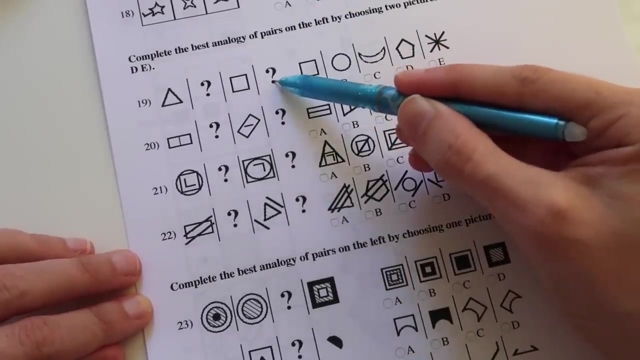 Onto the next page we have a few more of those examples, and then we have complete the best analogy of pairs by choosing two pictures from the right. So this means that we're saying, like a triangle is to something as a square is to something else, We need to establish a rule. 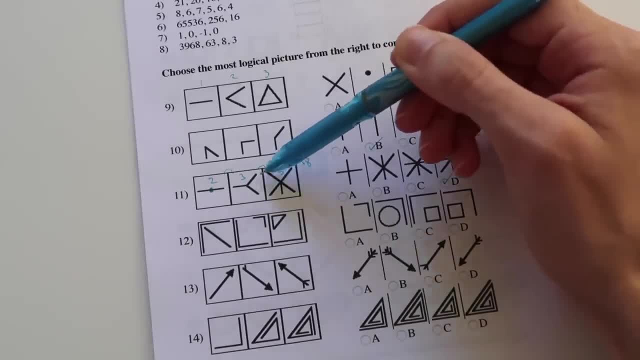 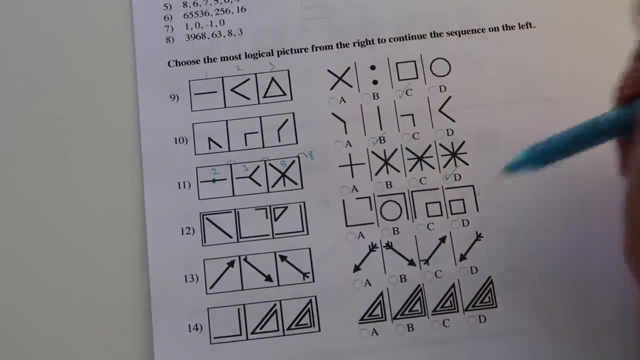 thinking that, oh, we're adding this V shape on every time, So you've added it here and then we've added it in here. If you added a V shape onto this one, you'd get C, but the answer that they give is D, and I agree that's a better way to do it. The rest of these problems are very similar. You're just 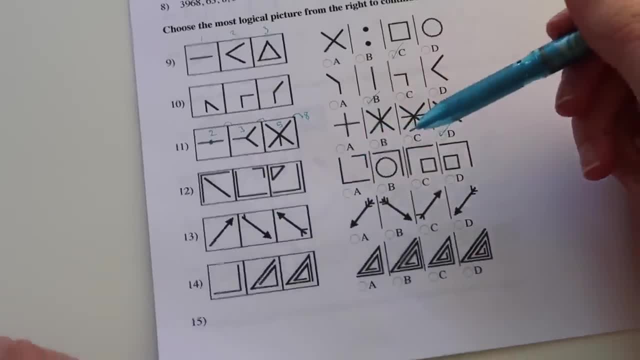 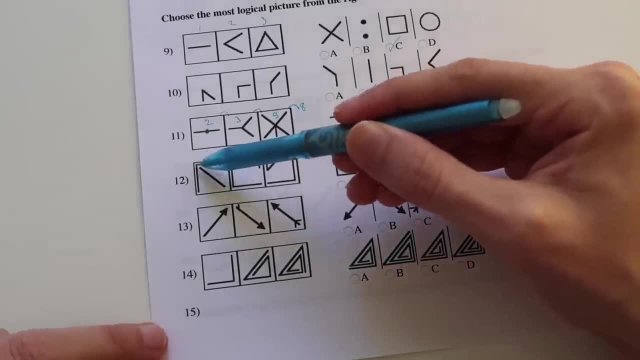 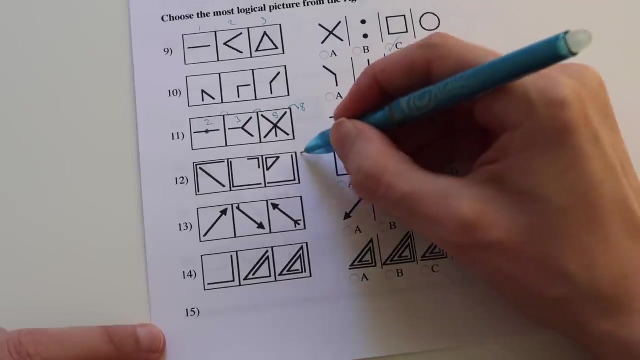 looking for, like slight changes or ways that these pictures evolve that are consistent. Sometimes different elements in the pictures evolve differently to other elements. like for number 12, we have this L which is going around the outside of the square counterclockwise, so we'd expect to. 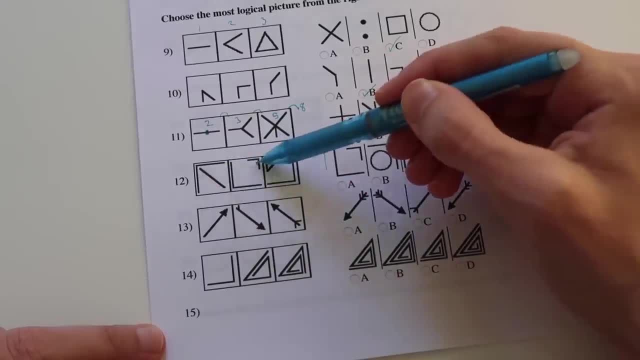 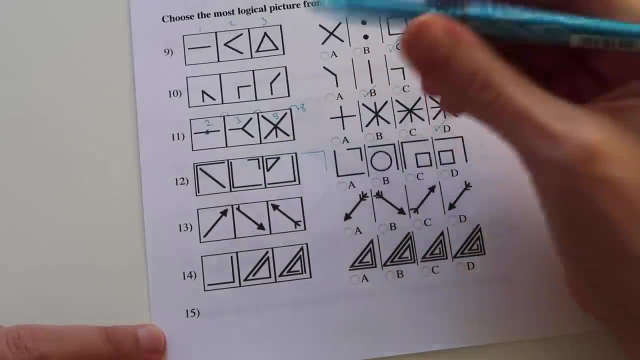 have a line like that in the next one and that's sort of independent from what's happening to the shape in here, which is that in like number nine the shape is increasing inside one every time. So we'd expect a square in the next one and a square and a line like that. that would give us D. 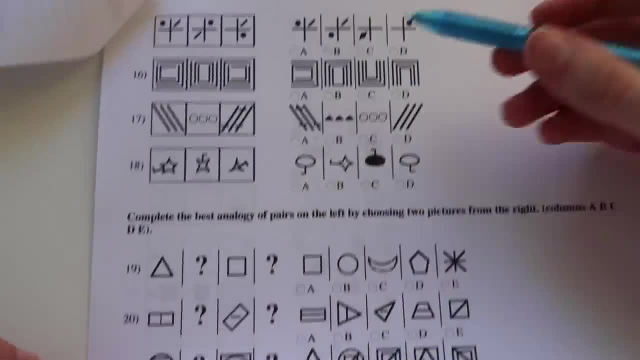 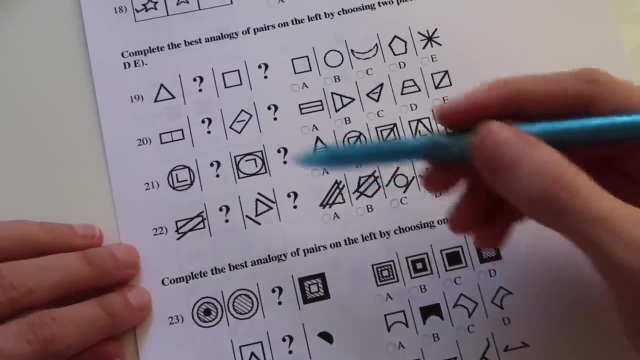 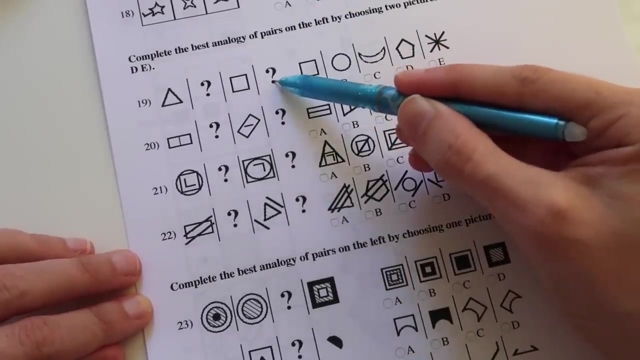 Onto the next page we have a few more of those examples, and then we have complete the best analogy of pairs by choosing two pictures from the right. So this means that we're saying, like a triangle is to something as a square is to something else, We need to establish a rule. 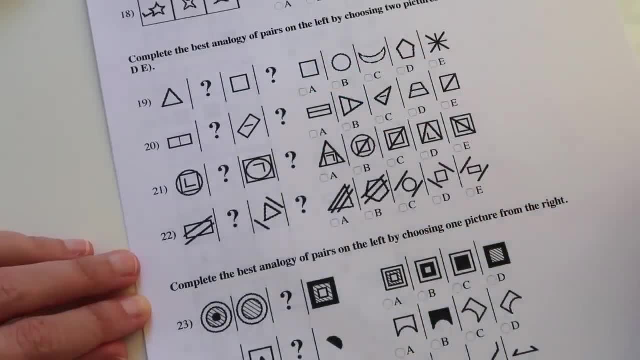 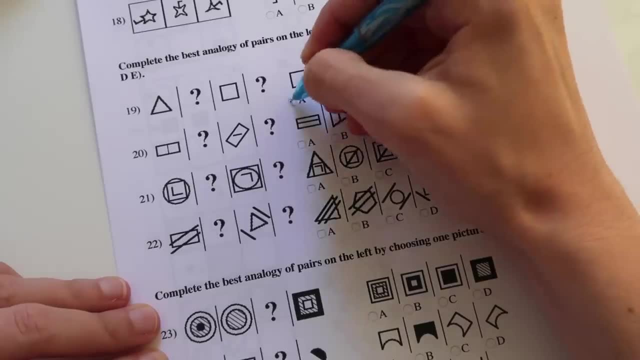 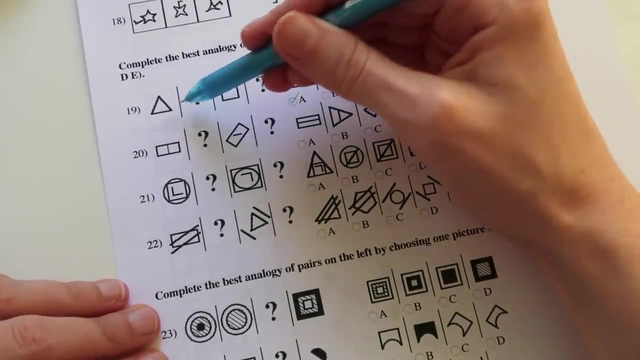 that links these two objects and also links these two objects In this case. again, it's to do with the sides of the shape. so a three-sided shape is to a, a square, as to a square is to a pentagon. They've both increased the side of the shape by one in each of these examples- Number 20 there could you. 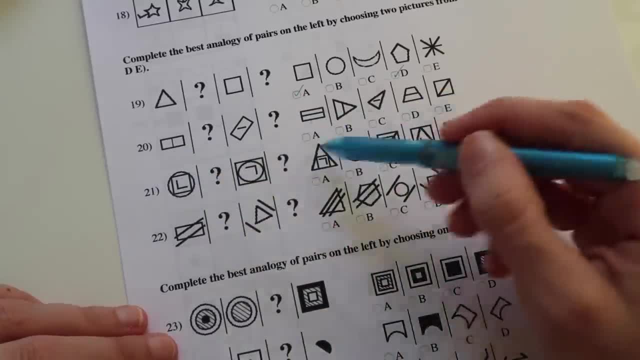 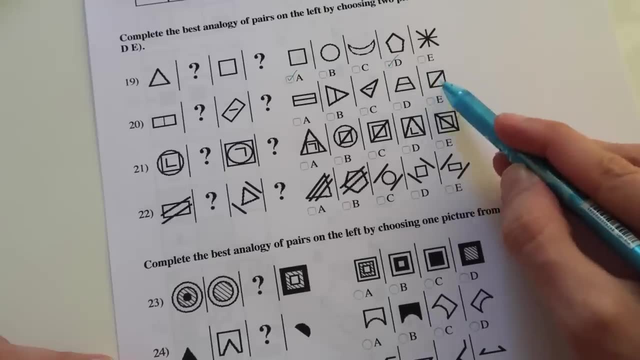 any number of ways that link these shapes, but we can look at the answers to get an idea of what's going on. So in the answers we have a rectangle, this shape and a square, but there's only one of each of those. so that kind of seems like it won't be consistent because, whatever happens, 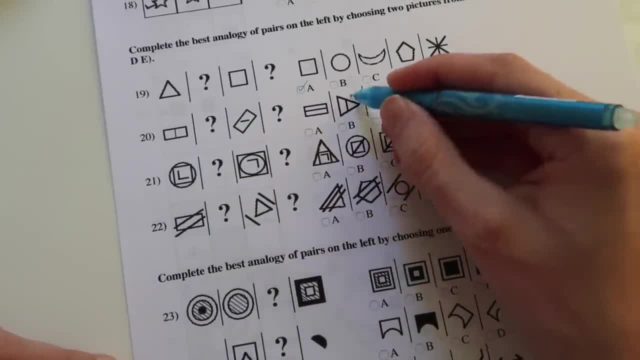 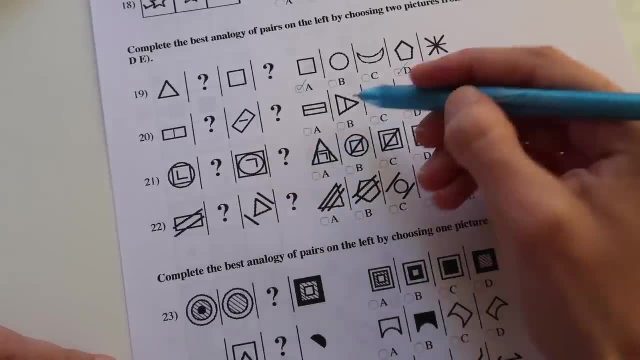 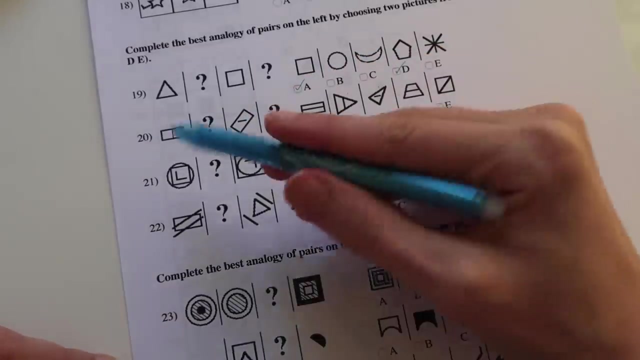 here needs to also happen here. What's similar is that B and C are both triangle type shapes, and how could they relate to these? Well, the little dash that's in the middle. this one has a vertical dash, this one has a horizontal dash. so if the rule is that the 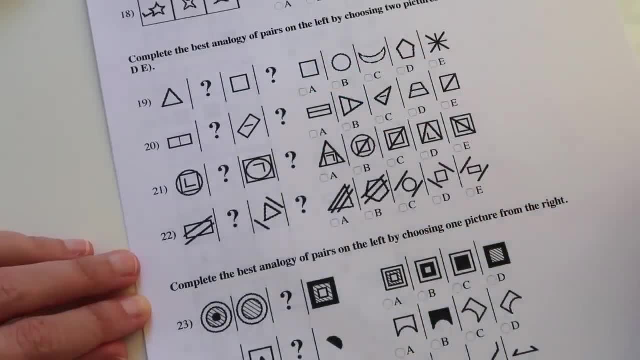 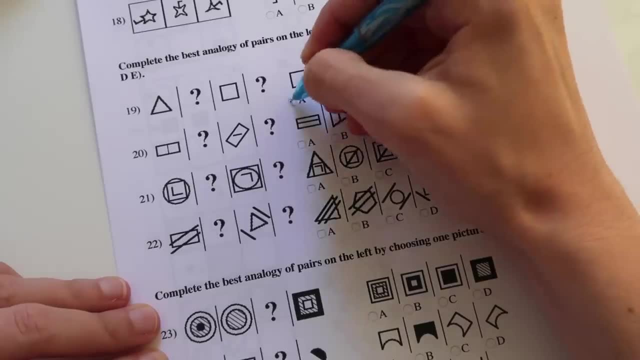 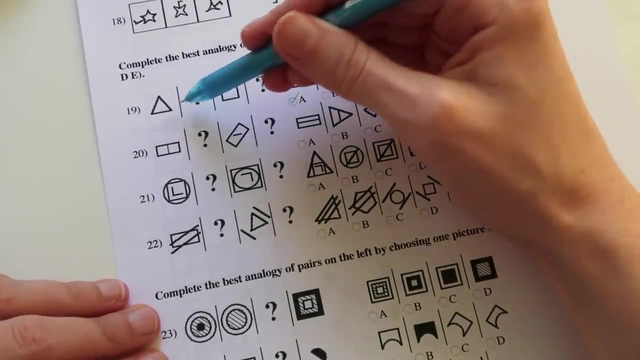 that links these two objects and also links these two objects In this case. again, it's to do with the sides of the shape. so a three-sided shape is to a, a square, as to a square is to a pentagon. They've both increased the side of the shape by one in each of these examples- Number 20 there could you. 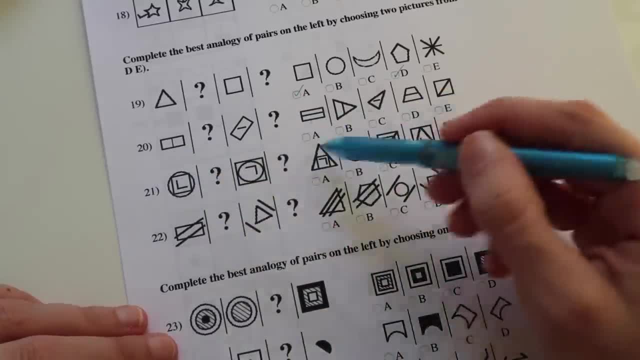 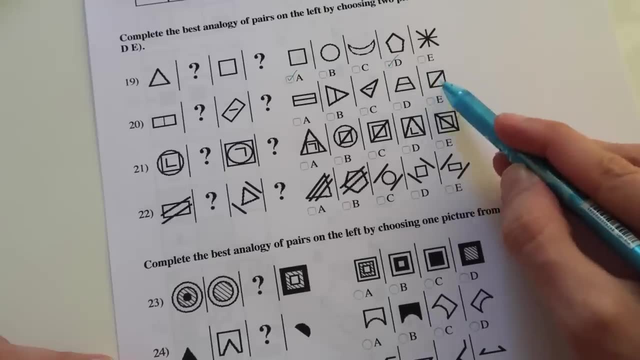 any number of ways that link these shapes, but we can look at the answers to get an idea of what's going on. So in the answers we have a rectangle, this shape and a square, but there's only one of each of those. so that kind of seems like it won't be consistent because, whatever happens, 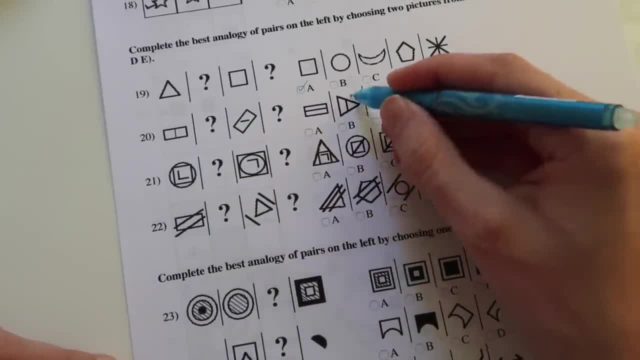 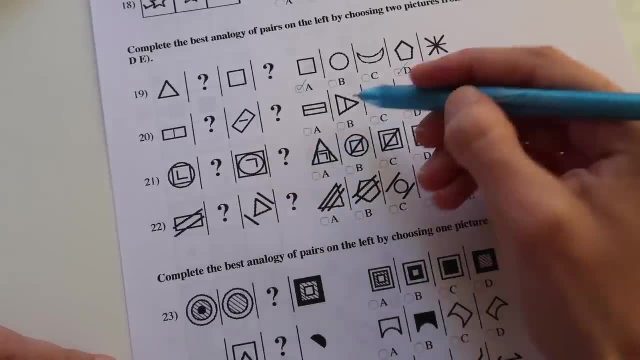 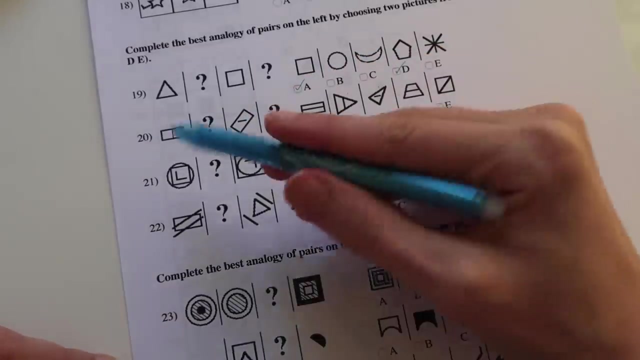 here needs to also happen here. What's similar is that B and C are both triangle type shapes, and how could they relate to these? Well, the little dash that's in the middle. this one has a vertical dash, this one has a horizontal dash. so if the rule is that the 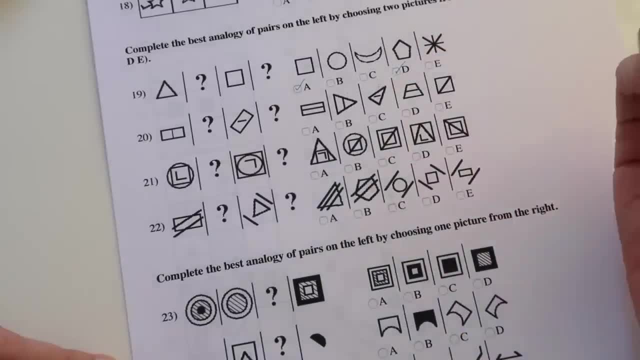 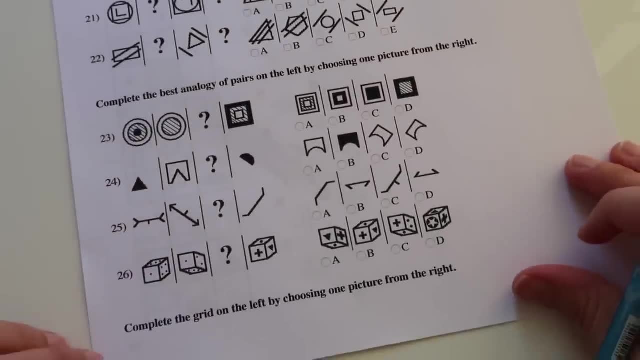 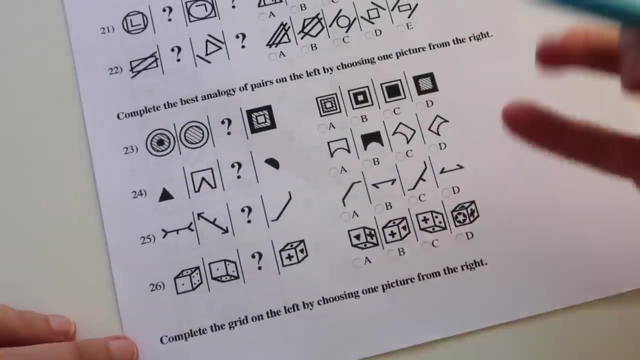 rectangle turns into a triangle and the dash stays the same, then it would make sense for B to go here and for C to be here. The next section is more analogy of pairs, except this time they essentially give us the rule. so they give us enough to work out the rule without referring. 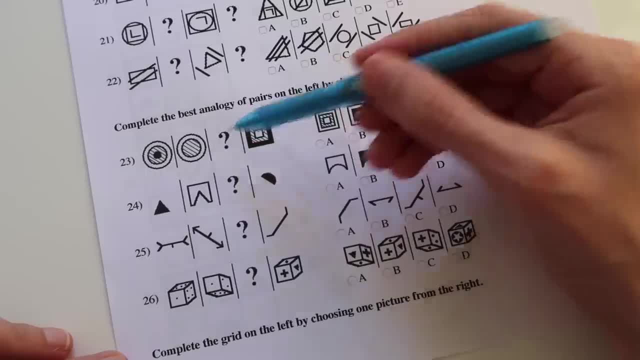 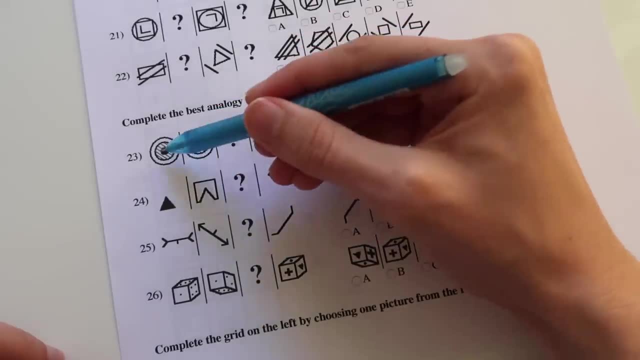 so much to the answers. to do that, Then we just need to apply that rule to find our one missing shape, This first one. I think this one's quite easy. what's happened between here and here? well, what's happened is this dot has gone missing in the middle. so if we apply that here, if we take away 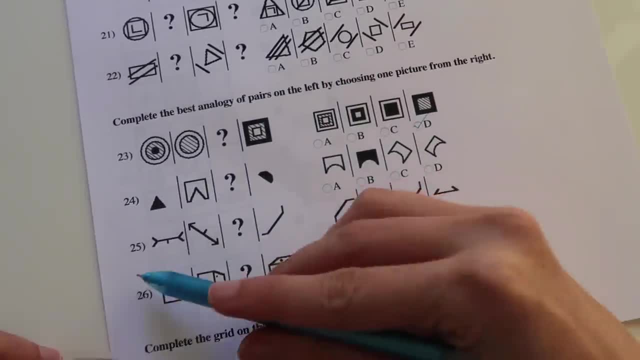 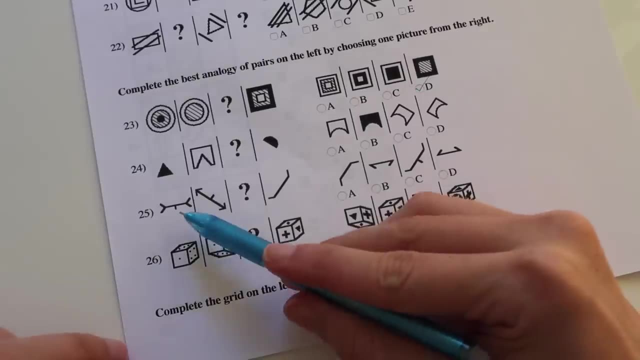 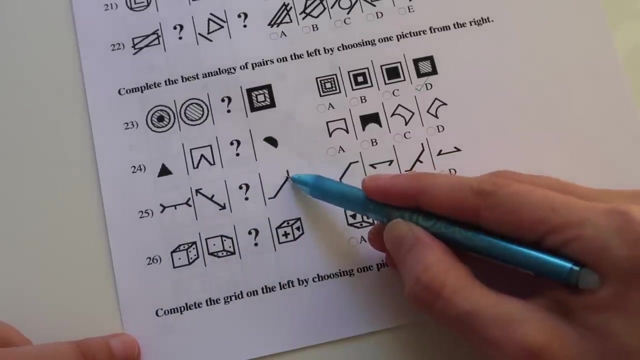 this little square in the middle, we'd end up with D. When we look at 25, we see that sometimes a familiarity with angles and rotations can help us out. so between here and here, you can first of all see that these arrowheads seem to get inverted. so this is what we are working with in the end. 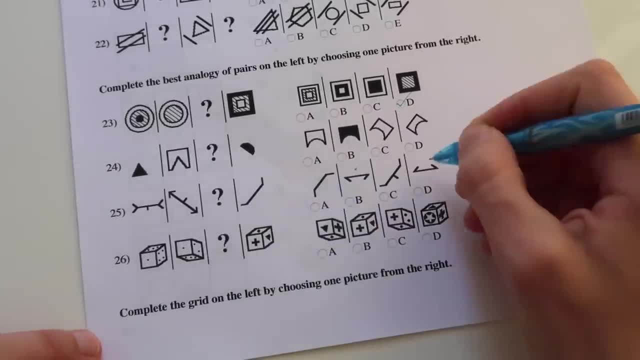 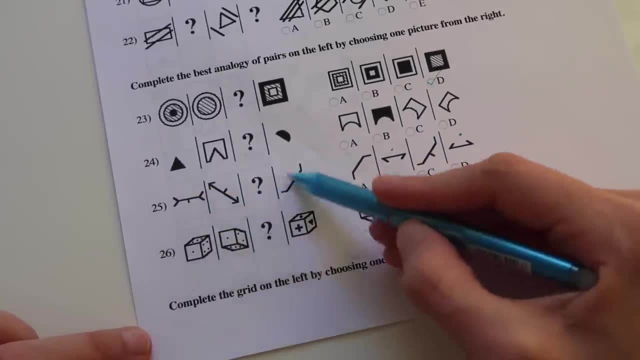 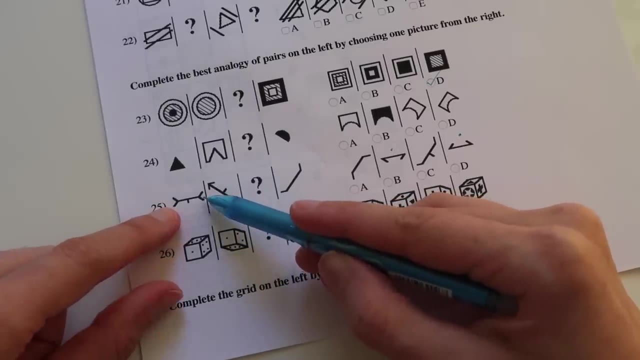 if you invert these little arrowheads, it looks like we want either B or D. but how do we work out which one of these? well, we have to figure out what rotation is happening here and apply it. in this case, This little dash helps. you know which way it's been rotating and actually it's going 90 plus. 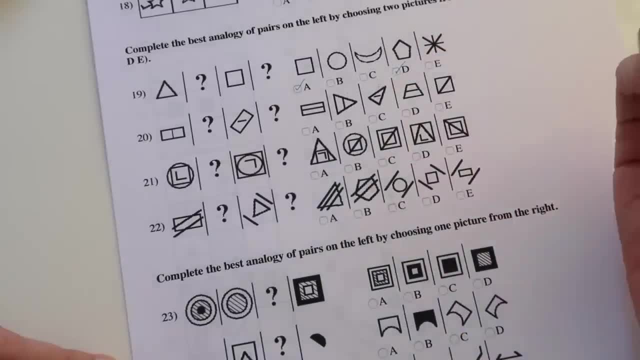 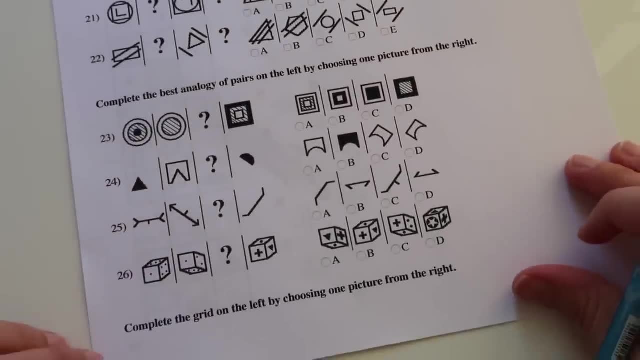 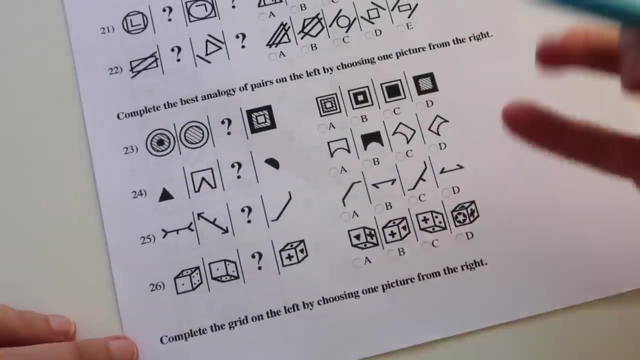 rectangle turns into a triangle and the dash stays the same, then it would make sense for B to go here and for C to be here. The next section is more analogy of pairs, except this time they essentially give us the rule. so they give us enough to work out the rule without referring. 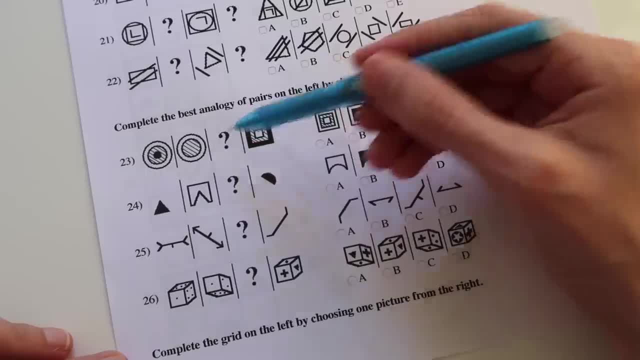 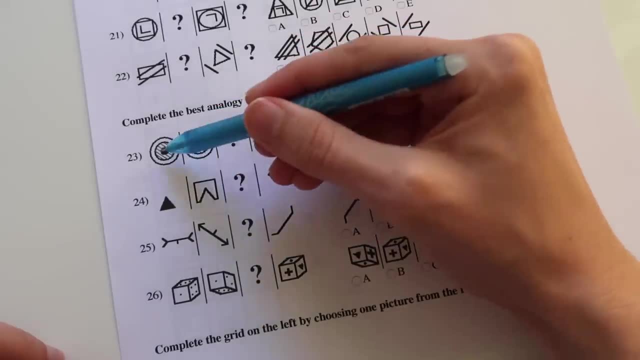 so much to the answers. to do that, Then we just need to apply that rule to find our one missing shape, This first one. I think this one's quite easy. what's happened between here and here? well, what's happened is this dot has gone missing in the middle. so if we apply that here, if we take away 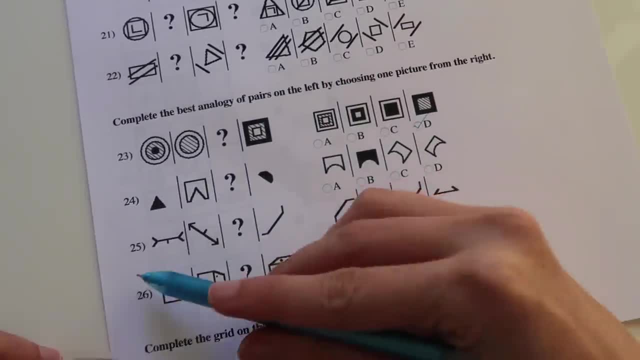 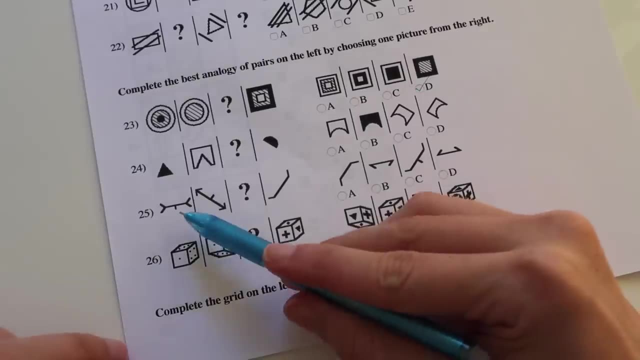 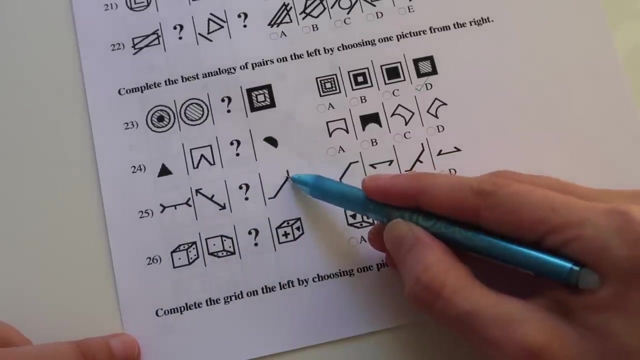 this little square in the middle, we'd end up with D. When we look at 25, we see that sometimes a familiarity with angles and rotations can help us out. so between here and here, you can first of all see that these arrowheads seem to get inverted. so this is what we are working with in the end. 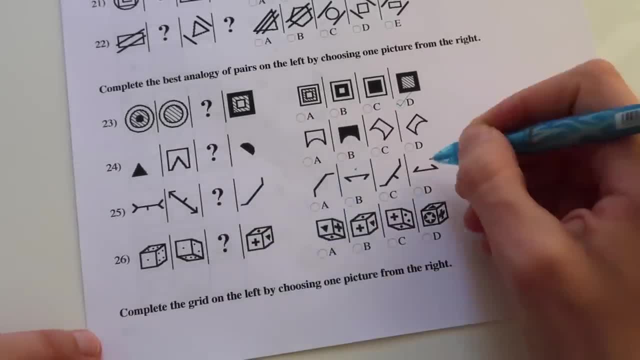 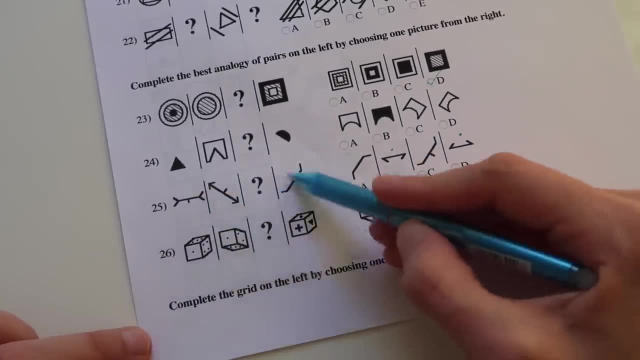 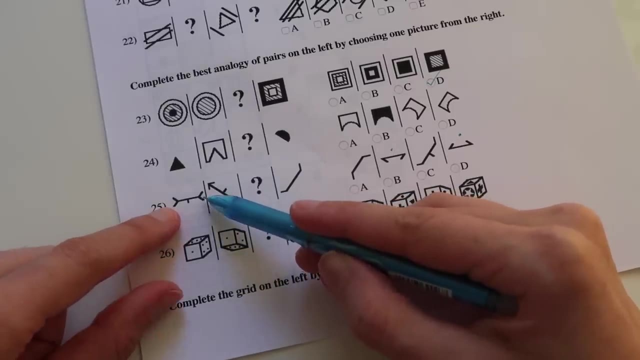 if you invert these little arrowheads, it looks like we want either B or D. but how do we work out which one of these? well, we have to figure out what rotation is happening here and apply it. in this case, this little dash helps. you know which way it's been rotating and actually it's going 90. 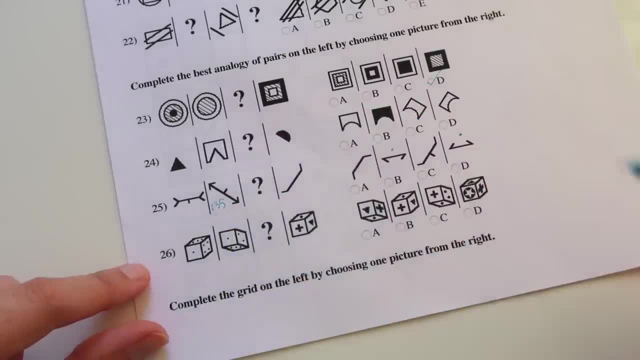 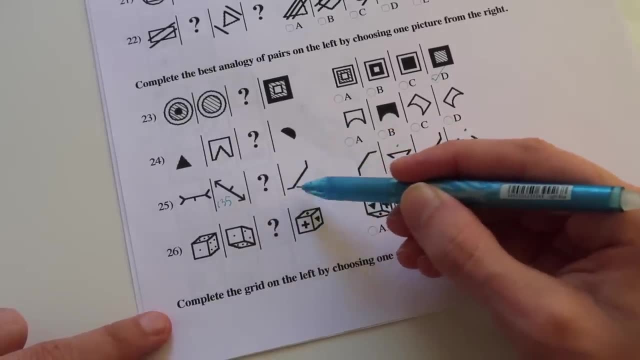 plus a little bit more. it's 135 degrees. for me, being able to store that number of 135 in my head when I'm starting to think about this, It helps me out. and if I didn't know, you know how angles work in a circle, maybe I'd find this. 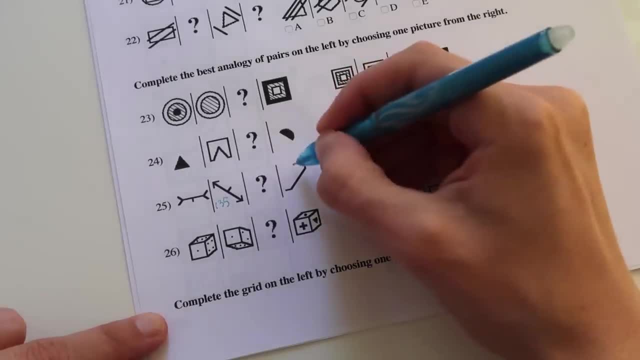 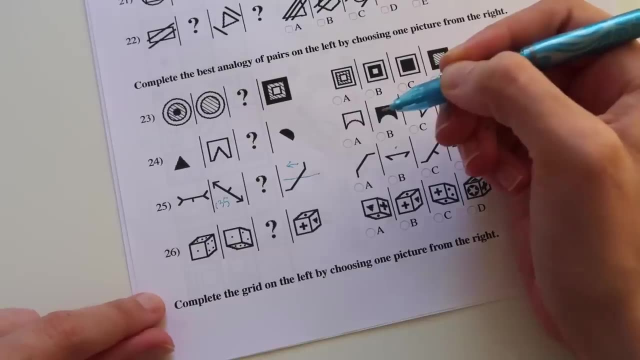 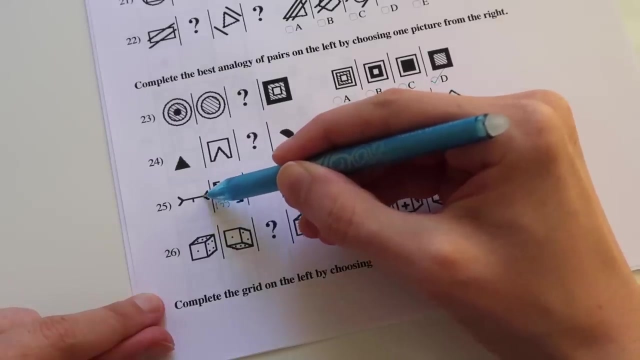 a little bit trickier. but if we do a 135 degree rotation on this answer here we'd be going this way, it would be 90 plus a bit more. we'd end up like this, with our little arrowheads like this, and then, if we invert them- which, looking at this, means taking them from being out to pointing- 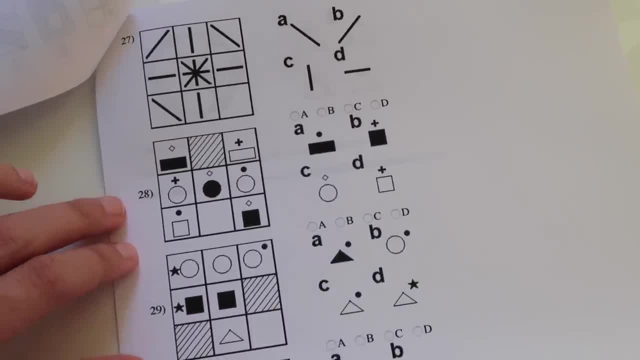 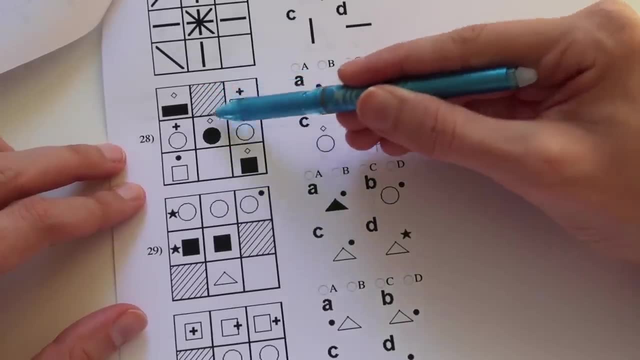 inwards, we would actually get B. This next page here is about completing the patterns on these words. we're trying to find the blank space, and then sometimes I've kind of blacked out one of the spaces, I guess, to make it trickier to find the pattern. the first one seems quite obviously to 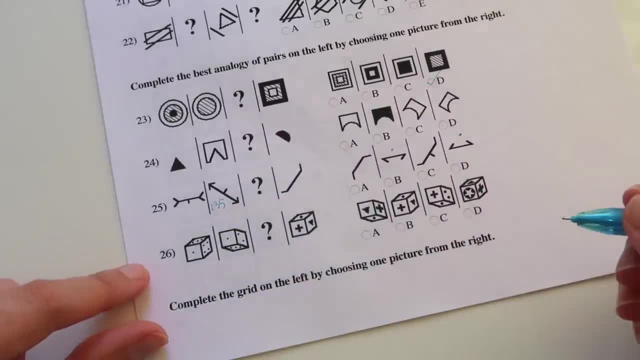 a little bit more. it's 135 degrees. For me being able to store that number of 135 in my head when I'm starting to think about this, how about if we just divide it up by three by three, and so you'll see that if this arrowhead is in the middle, that's the one that gets rotated, and the middle one gets rotated. so this little dash helps. you know which way it's been rotating. and actually it's going 90 plus a little bit more. it's 135 degrees. for me being able to store that number of 135 in my head when I'm starting to think about this. 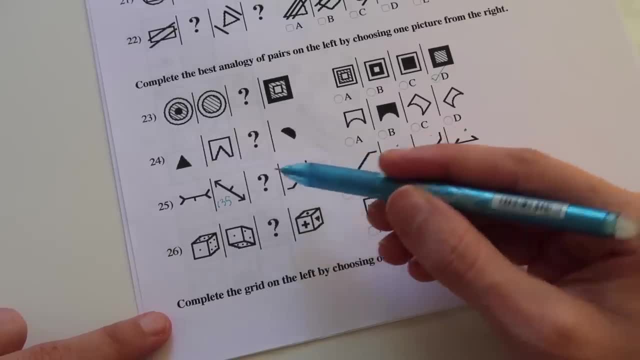 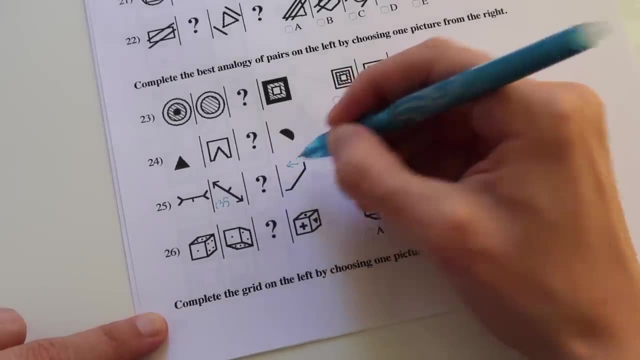 helps me out. and if I didn't know, you know how angles work in a circle, maybe I'd find this a little bit trickier. but if we do a 135 degree rotation on this answer here we'd be going this way: it would be 90 plus a bit more. we'd end up like this, with our little arrowheads like this: 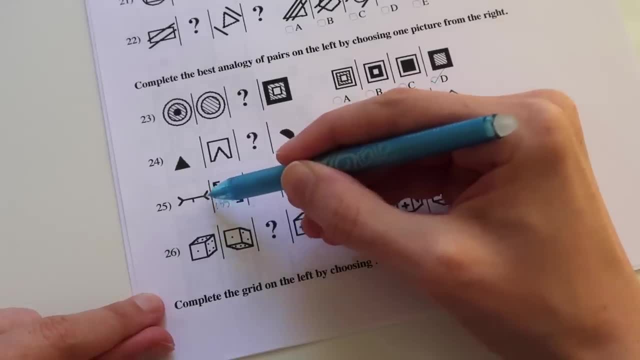 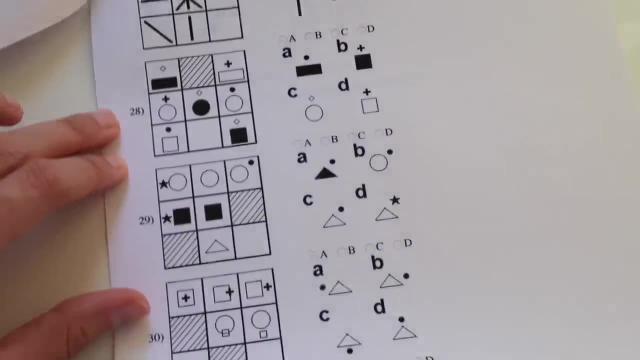 and then if we invert them- which looking at this, means taking them from being out to pointing inwards- we would actually get b. This next page here is about completing the patterns on these grids. we're trying to find the blank space, and then sometimes I've kind of blacked out one of 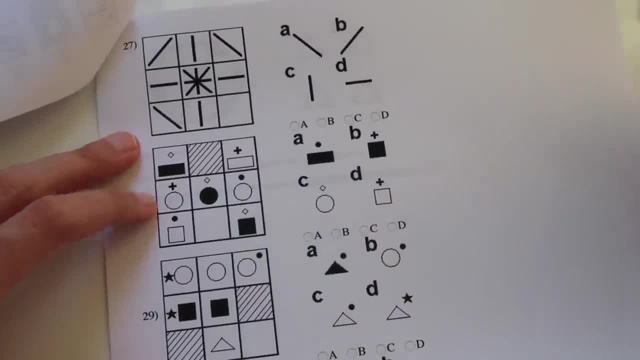 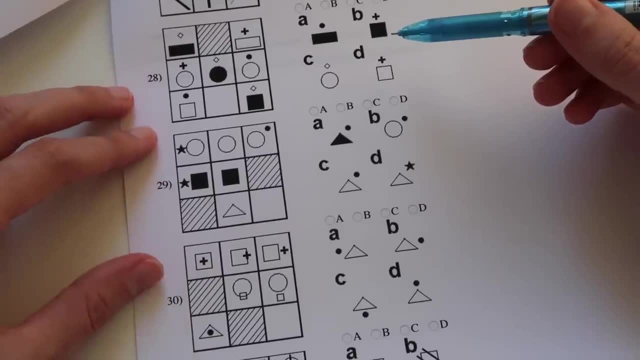 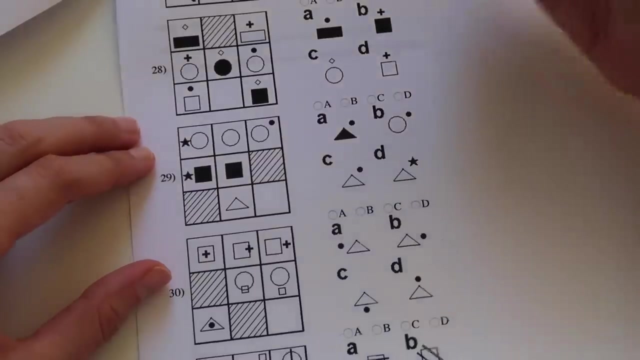 the spaces, I guess to make it trickier to find the pattern. The first one seems quite obviously to be like this, which is going to be b, and then pretty much all the rest of them have the same sort of pattern. First of all, look for shapes that are similar, between rows and columns, for example. 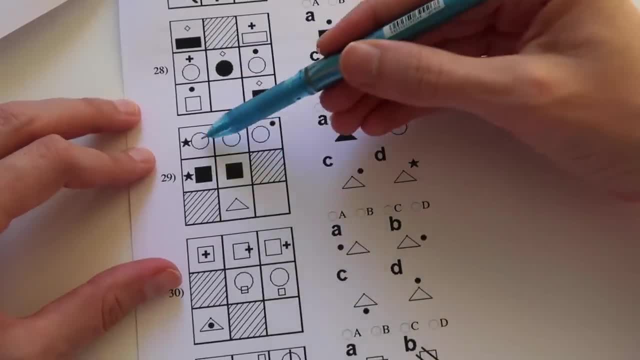 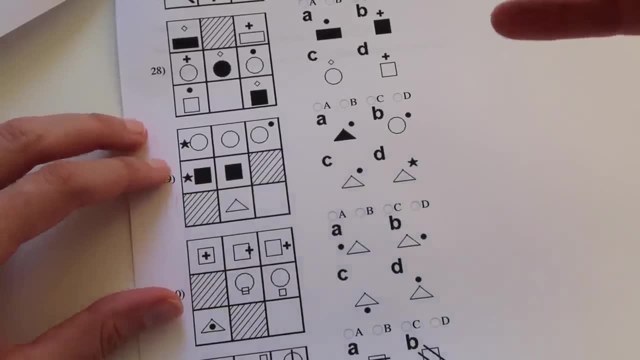 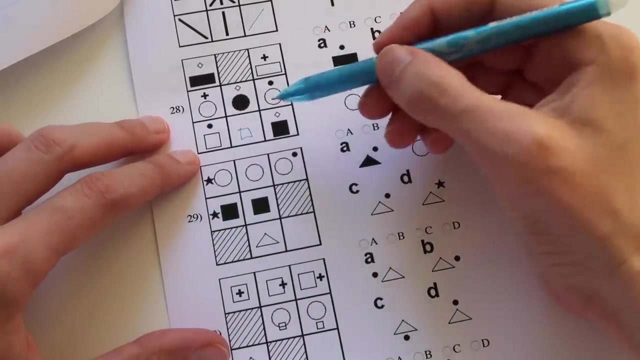 rectangles, circles, squares, and then, down here, circles, squares, triangles. There's often rules that link all the columns or rows by some common theme. In this example, we're going to be expecting a square down here to complete that rows rule, and then what color is it going to be? Well, we've only 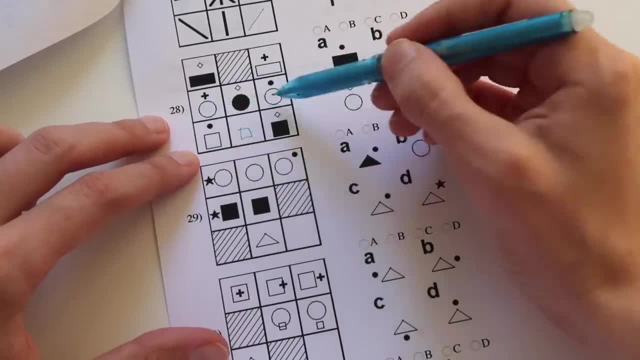 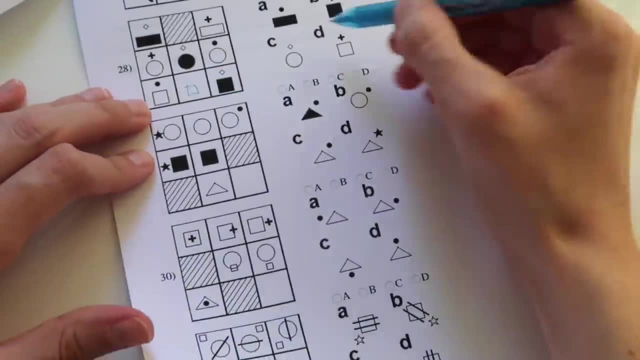 really got full information on this middle line and it looks like there will be two white and one black, so we can expect this one to be white, because we've got a black here and a white here. There is only one answer, which is a square that is white, and that would be d Very similar for 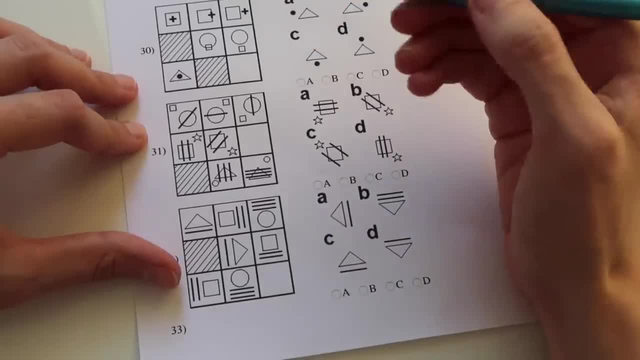 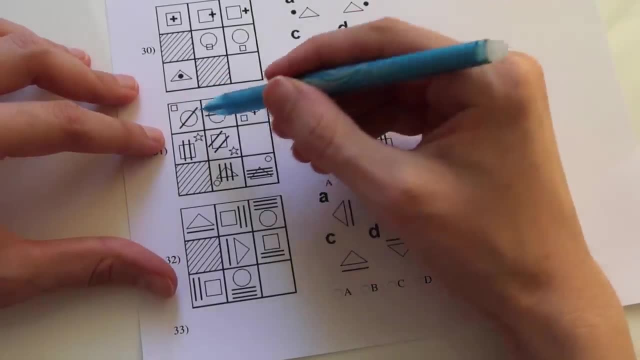 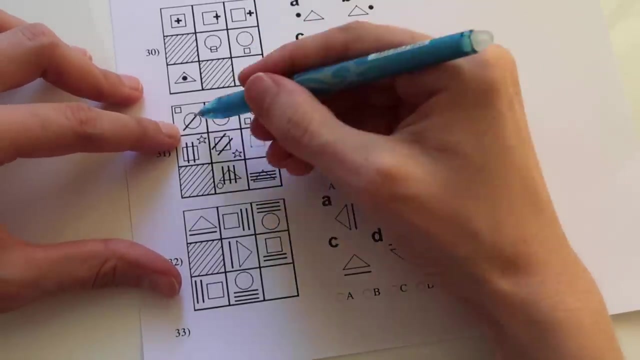 the next two, 31, may be slightly trickier. We have to isolate each element here. so we have shapes, lines and then little symbols. Looking at the shapes, we've got circles, squares, triangles, so we'd expect a square in here. Let's look at the lines now Between this one and this one. 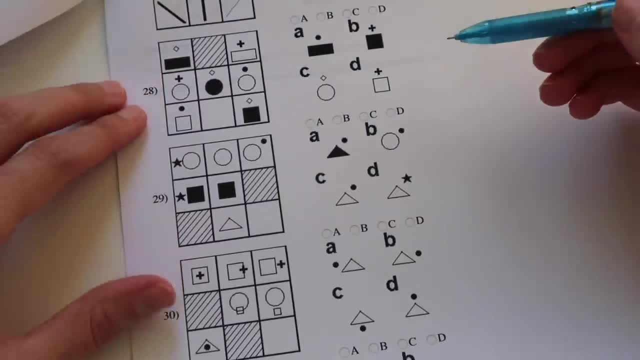 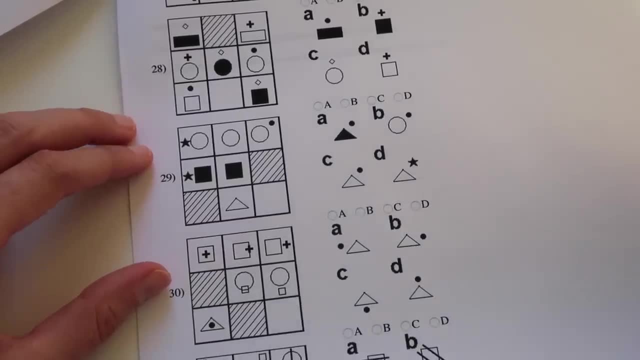 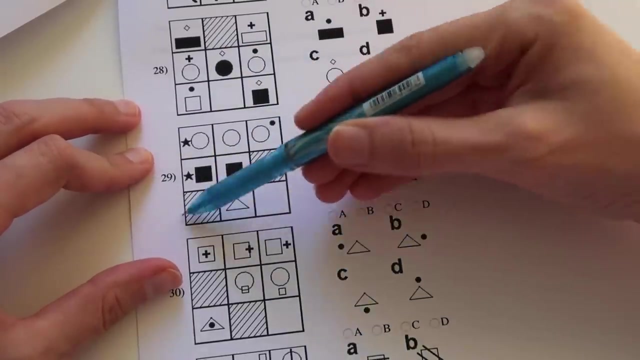 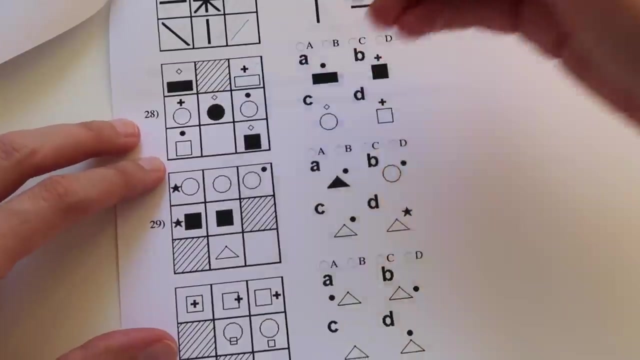 be like this, which is going to be B, and then pretty much all the rest of them have the same sort of pattern. first of all, look for shapes that are similar between rows and columns, for example, rectangles, circles, squares, and then down here, circles, squares, triangles. there's often rules that link all the columns or rows by some common theme. in this example, we're 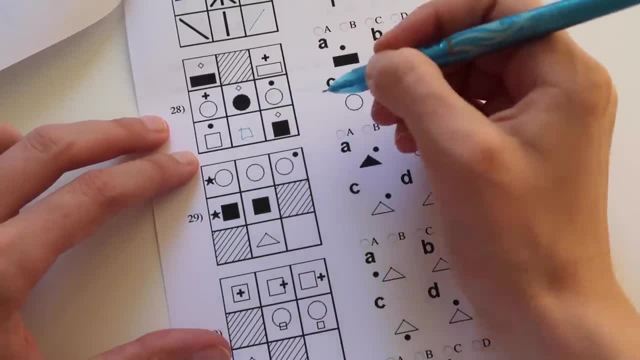 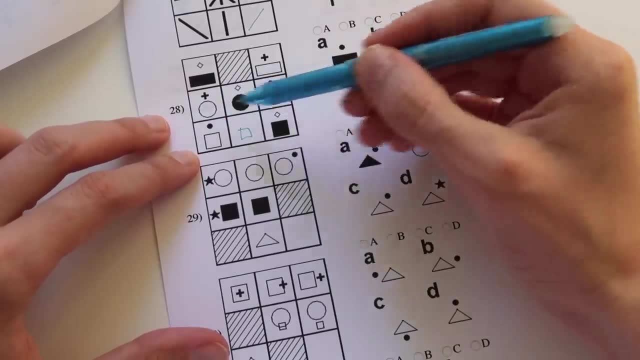 going to be expecting a square down here to complete that rows rule. and then, what color is it going to be? well, we've only really got full information on this middle line and it looks like there will be two white and one black. so we can expect this one to be white because we've got a 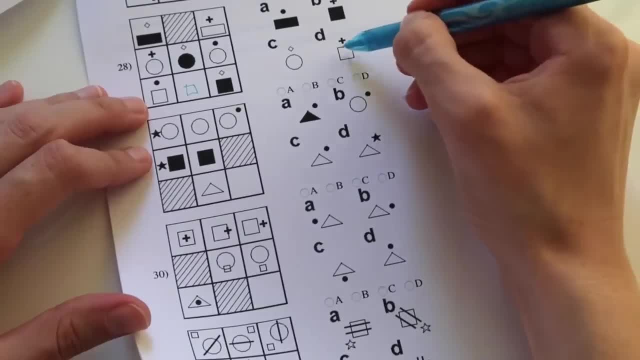 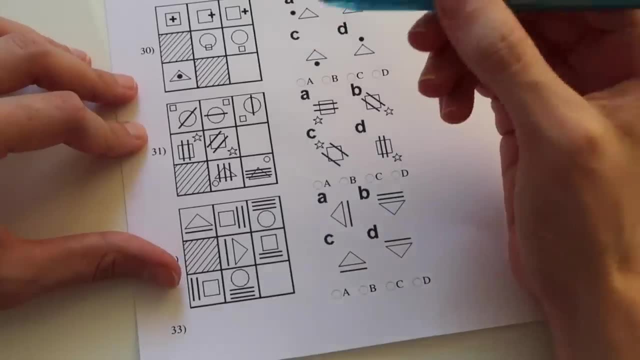 black here and a white here. there is only one answer, which is a square that is white, and that would be D, Very similar. for the next two, 31, may be slightly trickier. we have to isolate each element here, so we have shapes, lines and 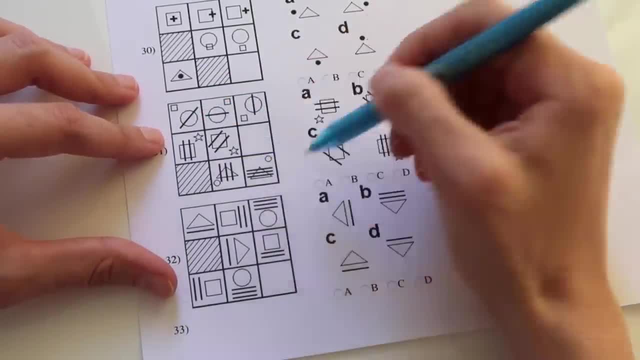 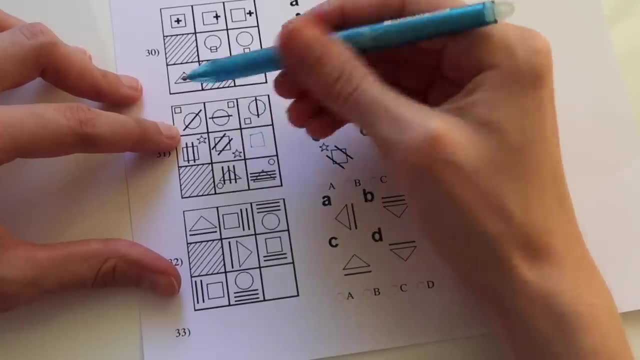 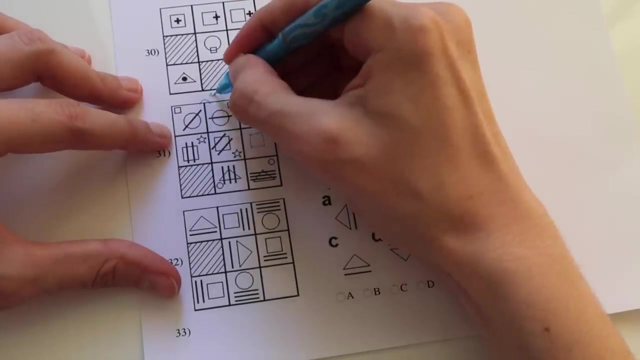 then little symbols. looking at the shapes, we've got circles, squares, triangles, so we'd expect a square in here. let's look at the lines now between this one and this one, we have going on a very small rotation. looks like a 45 degree rotation of this line, so 45 and that's consistent between these two. 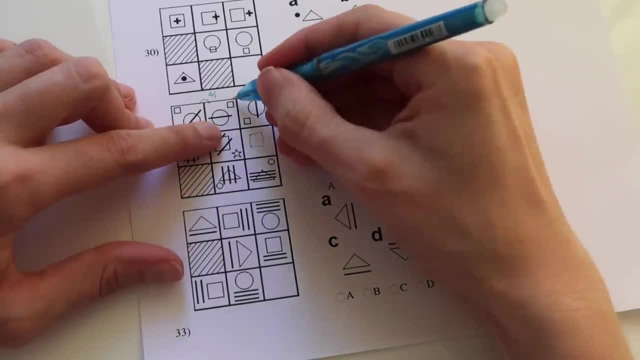 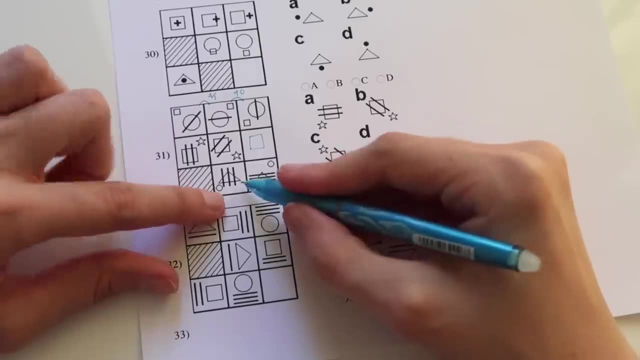 as well. that's another 45. Then between this column and this column it's no longer a 45 degree rotation, now it is 90 degrees. okay, and that's seen down here too. these lines flip 90 degrees, so we can expect a 90 degree rotation. 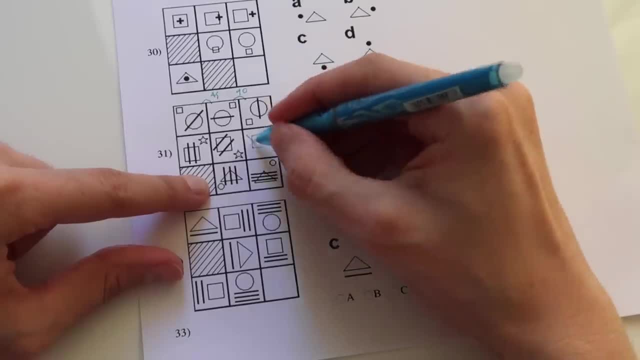 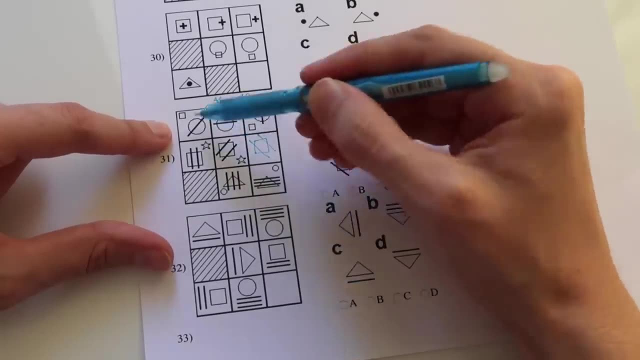 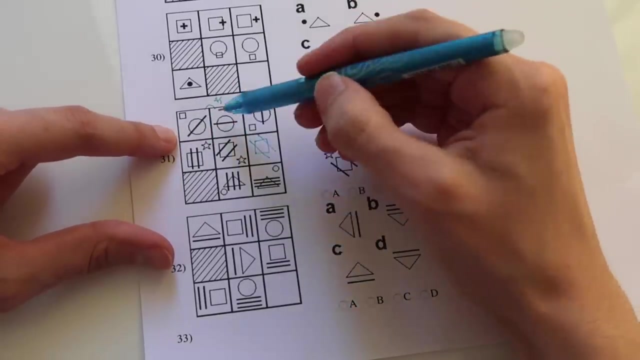 between these lines and here that would give us lines like this. so now we need to look at the little symbols, and between this column and this column, from looking at the square and the star, looks like the shapes are moving clockwise around the corners. they move one spot at a time. however, that changes again between the second and third columns and we 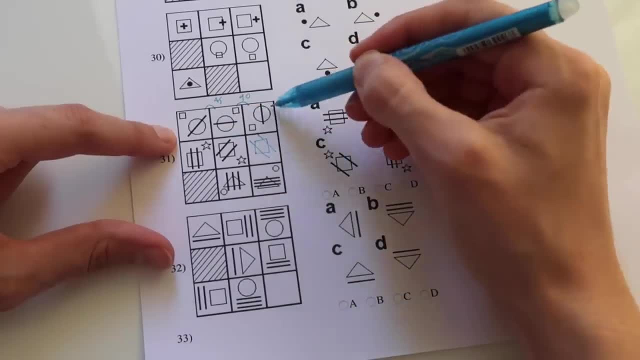 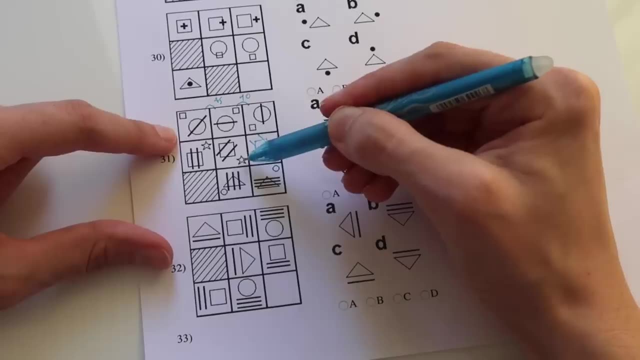 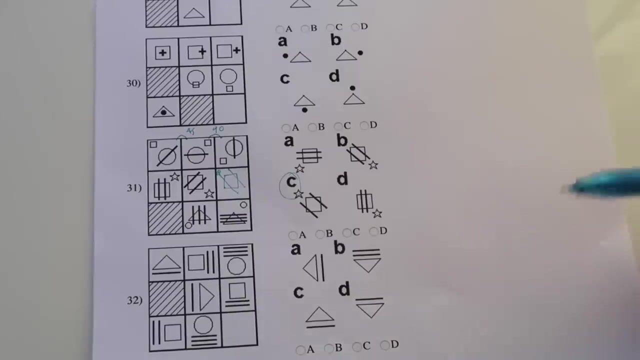 see that the shape now moves. well, it advances two corners at a time, so it advances all the way down to here. we see that as well with the circle goes to here. so if we advance the star two places, we'd be one, two, we'd expect our star up here and that would give us answer C. Some of these visual. 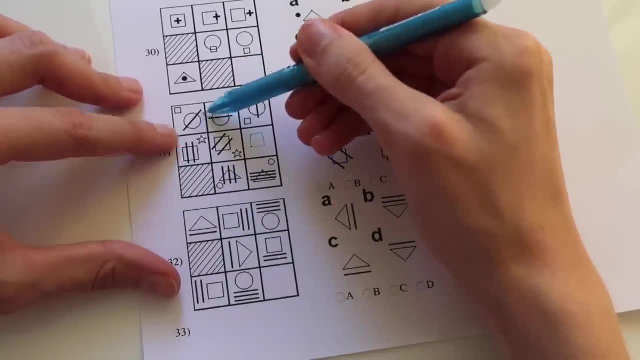 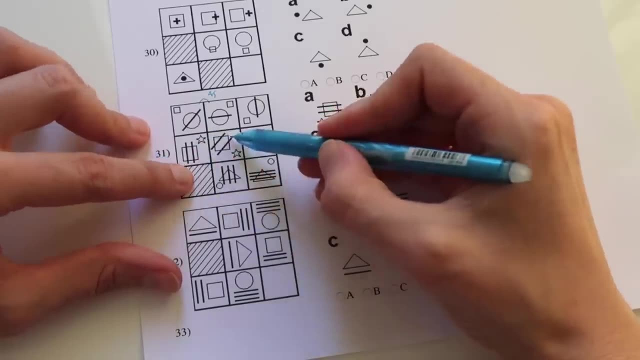 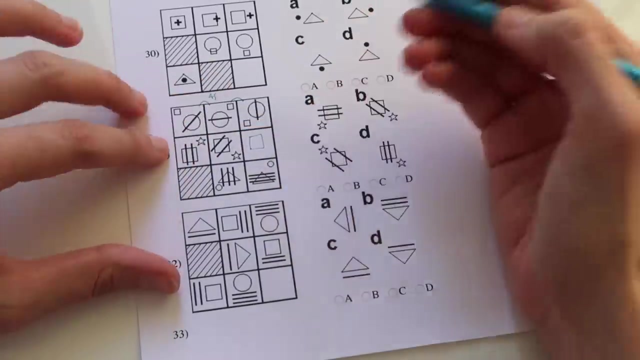 we are going on. a very small rotation Looks like a 45 degree rotation of this line, So 45, and that's consistent. between these two as well, That's another 45. Then, between this column and this column, it's no longer a 45 degree rotation, Now it is 90 degrees. Okay, and that's. 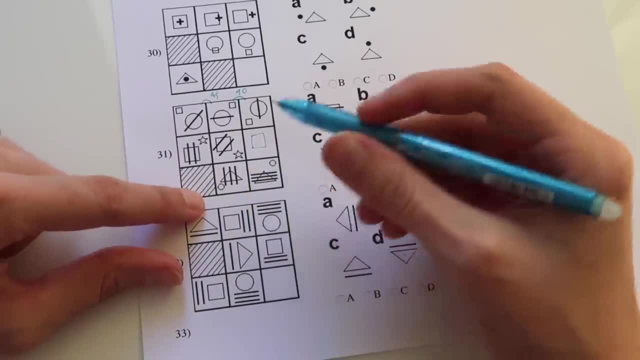 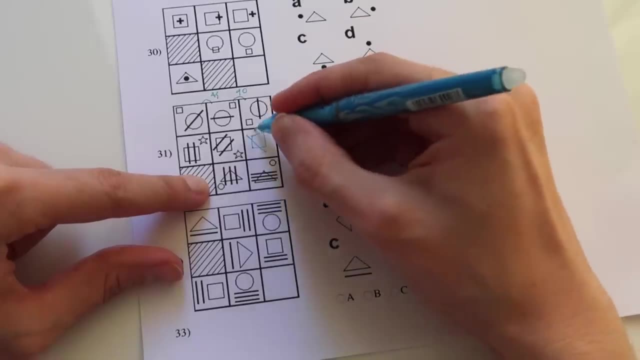 seen down. here too, These lines flip 90 degrees, So we can expect a 90 degree rotation between these lines, and here That would give us lines like this. So now we need to look at the little symbols, and between this column and this one we've got a 45 degree rotation of this line. 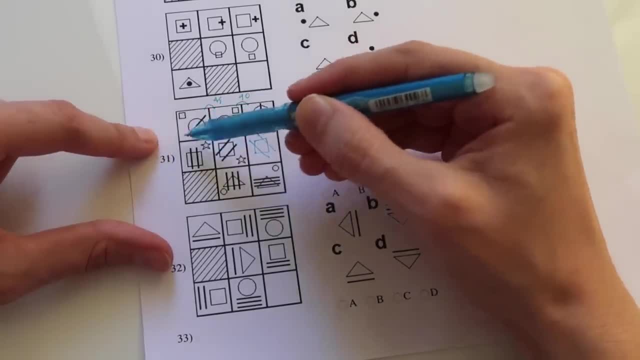 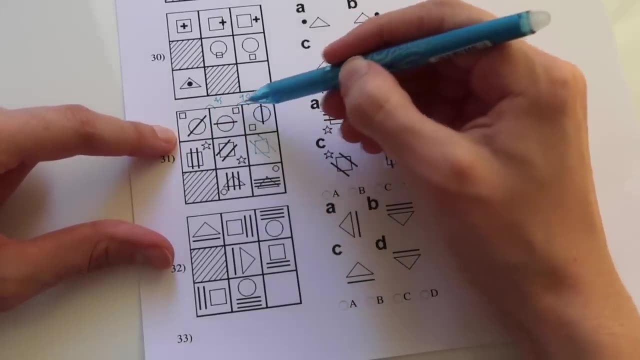 From this column, from looking at the square and the star, looks like the shapes are moving clockwise around the corners and they move one spot at a time. However, that changes again between the second and third columns and we see that the shape now moves. well, it advances. 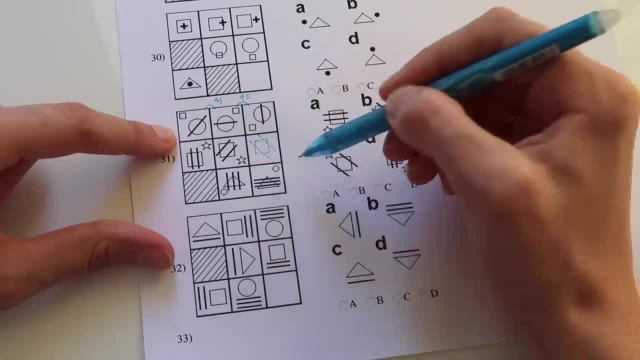 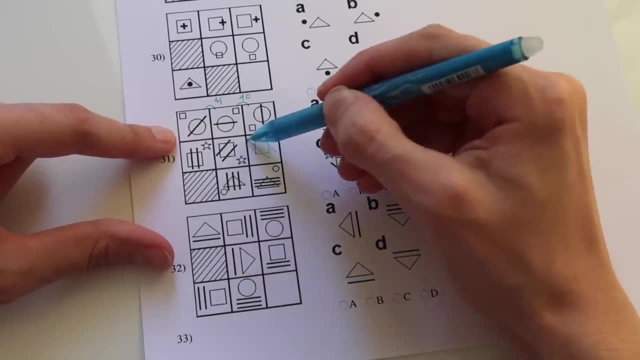 two corners at a time. So it advances all the way down to here. We see that as well with the circle goes to here. So if we advance the star two places, we'd be 1, 2.. We'd expect our star up here and that would give us answer c. 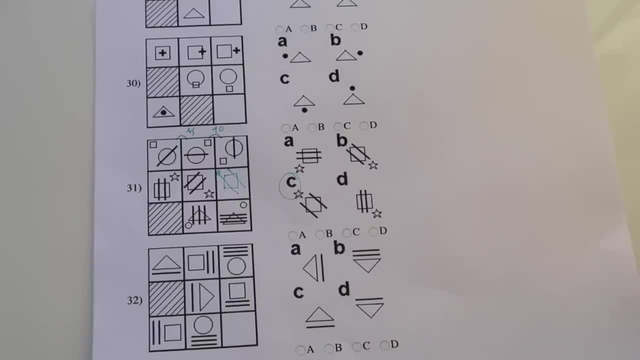 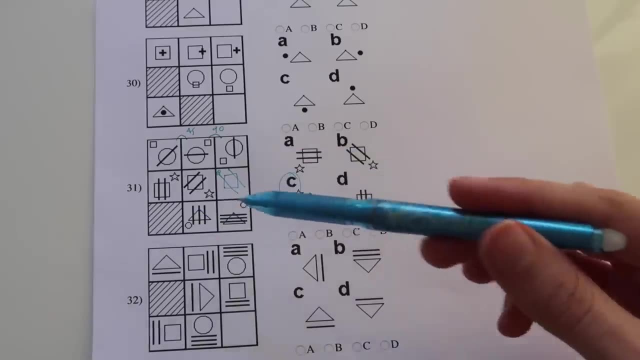 These visual patterns. I feel they can be slightly overwhelming to first look at because it seems like there are so many random moving parts. But try to isolate each element and what it's doing. Sometimes it's working completely independently of other elements, It does seem. 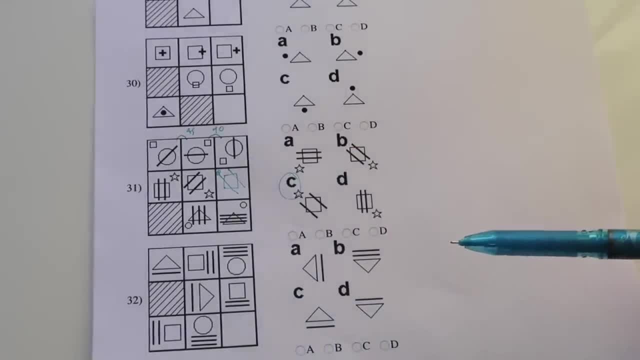 a bit strange that we're using these very abstract little puzzles to try and measure something as complex as intelligence. Our world is so complex and we're trying to measure what's going on in the world through these little patterns, And does that mean that everything in life comes down to just recognising patterns? Well, maybe that is a part of it. 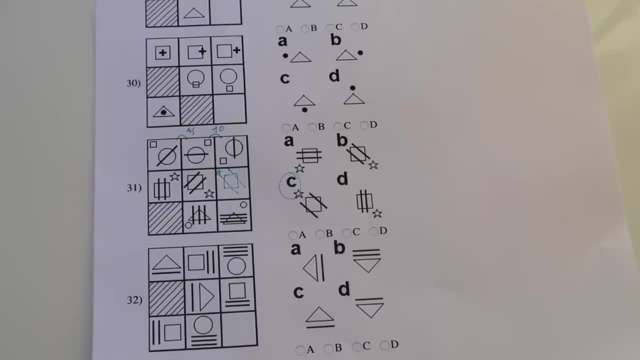 Maybe if being able to see how something evolves and works out from a little bit of evidence that you've got already, maybe that is what intelligence is, That you can identify those things. I guess I'm not totally sold on IQ tests, but it's interesting to just have a little look. 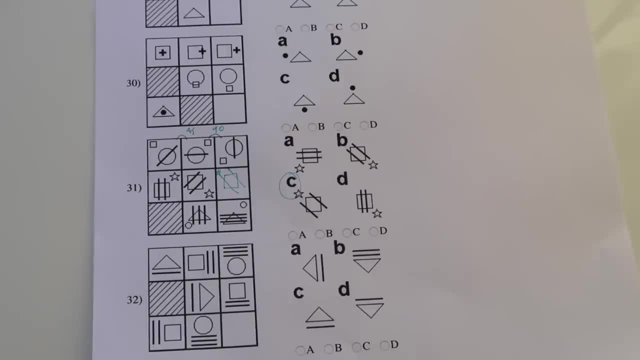 at what they're asking us. If you do well, you know it can be a good way to make you feel good, To sort of fluff up your ego a little bit, And if you do poorly, when you can always say you know these things. 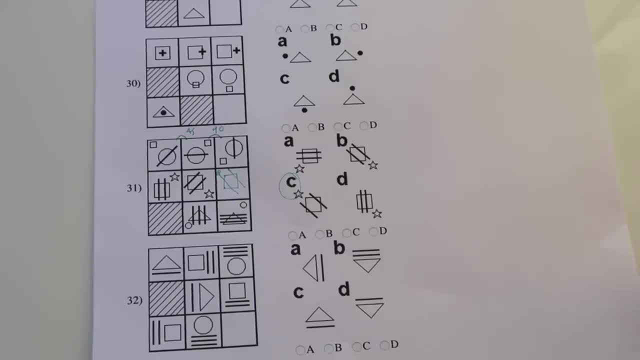 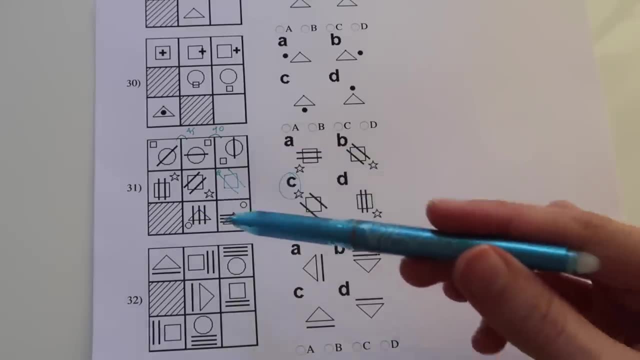 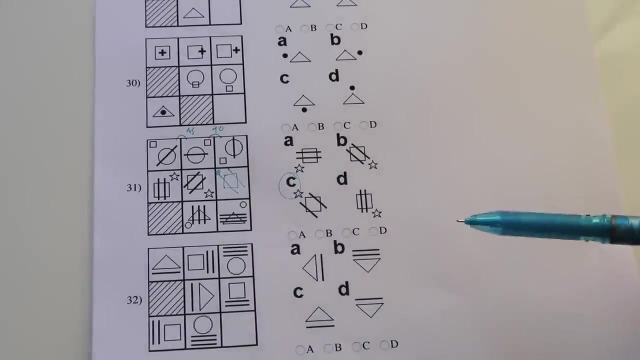 patterns. I feel they can be slightly overwhelming to first look at because it seems like there are so many random moving parts. but try to isolate. you know each element and what it's doing. sometimes it's working completely independently of other elements. it does seem a bit strange that we're using these. 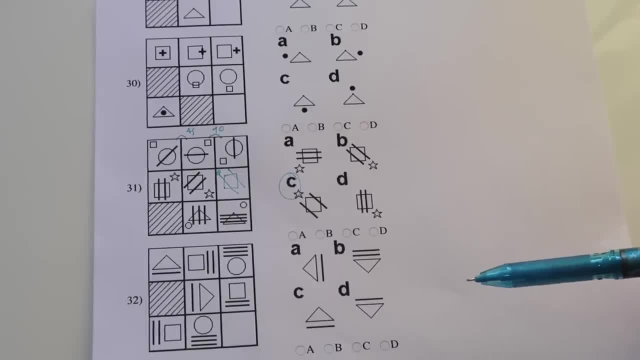 very abstract, little, you know, puzzles, to try and measure something as complex as intelligence. our world is so complex and you know we're trying to measure our interaction with it through these little patterns, and does that mean that everything in life comes down to just recognizing patterns? well, maybe that is a part of it. maybe if being able to see how something 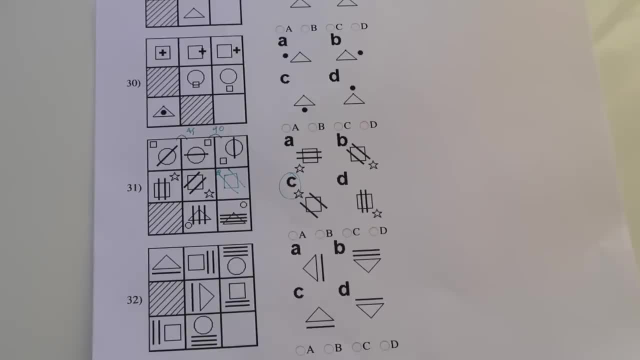 evolves and works out. um, from a little bit of evidence that you've got already, maybe that is what intelligence is, that you can identify those things. I guess I'm not totally sold on IQ tests, but it's interesting to just have a little look at what they're asking us. I guess, with these sorts of 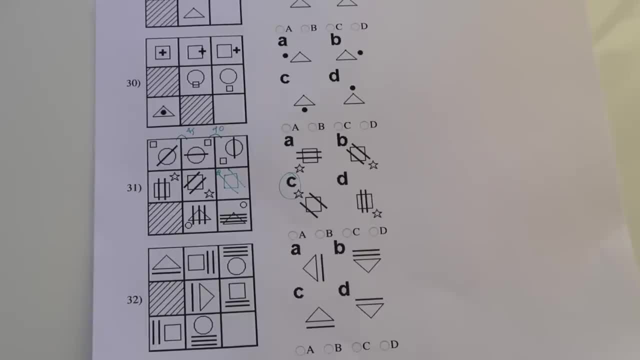 tests. if you do well, you know it can be a good way to make you feel good, to sort of fluff up your ego. And if you do poorly, when you can always say you know these things are sort of subjective. you know How can you measure intelligence with a test. There's a few more patterns here that you can try. There's one. 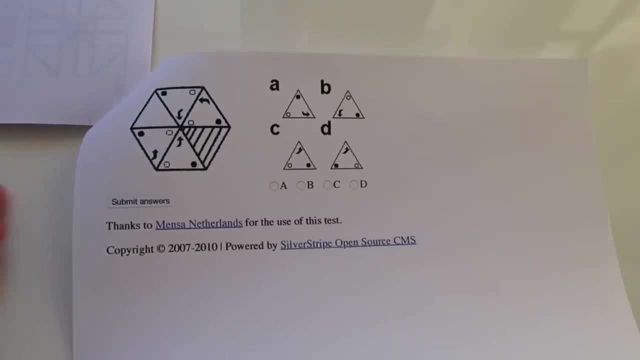 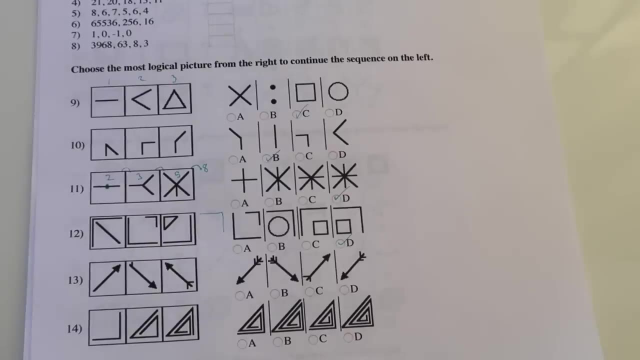 more on this following page. If you found it a breeze, maybe you even want to try out for Mensa, But I hope it was a little bit of insight into what's going on here And thanks for watching. If you were curious about this shirt, it is some merch from Black Pen- Red Pen. 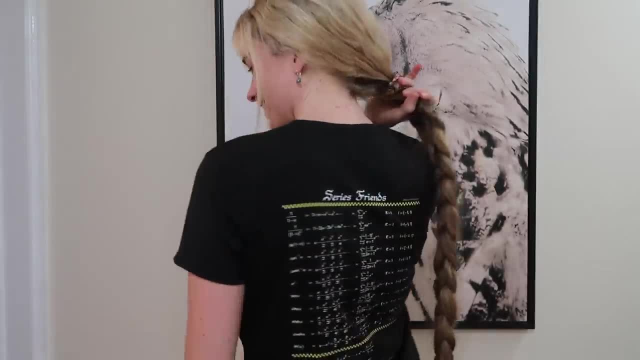 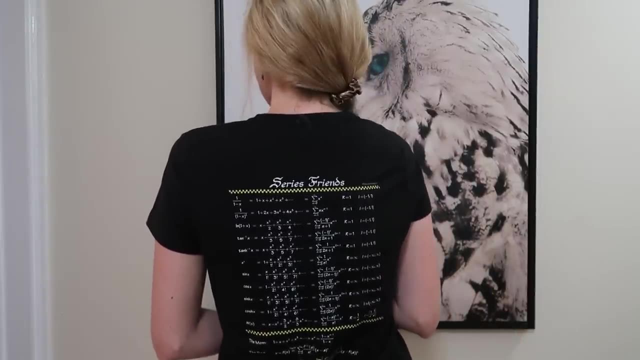 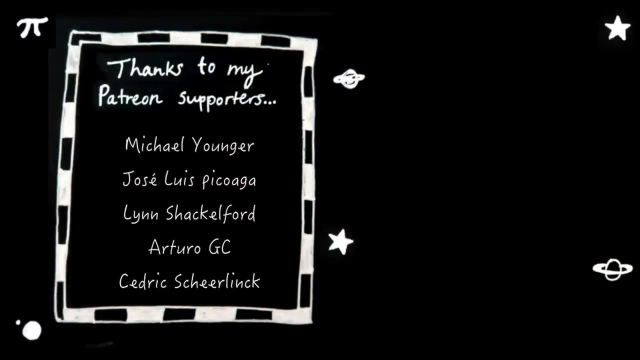 He makes awesome math videos and I'll put a link in the description to his channel and I'd encourage you to check him out. You probably can't wear this shirt to an exam, but it's a pretty cool one You.